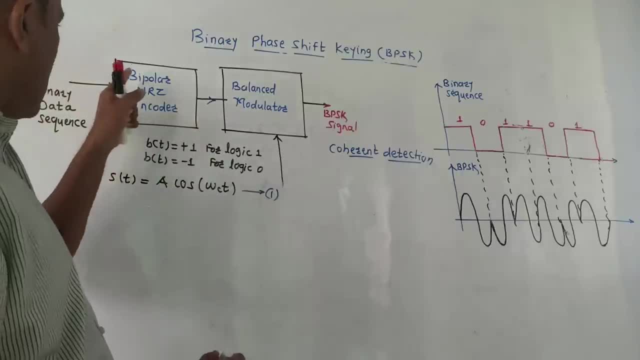 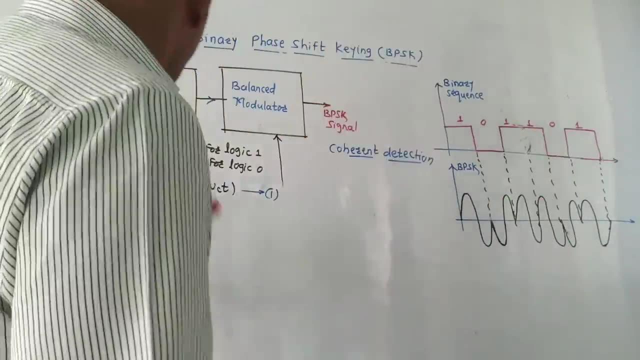 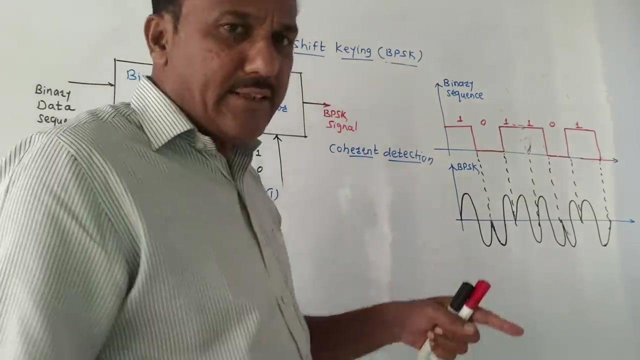 Alright, Now let us first talk about the block diagram of generator of BPSK. It is also called BPSK transmitter Input side. I have written binary data sequence, So incoming data is in the form of binary. That means logic 0 and logic 1.. 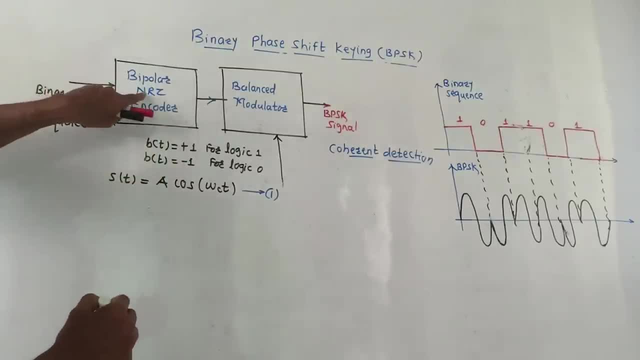 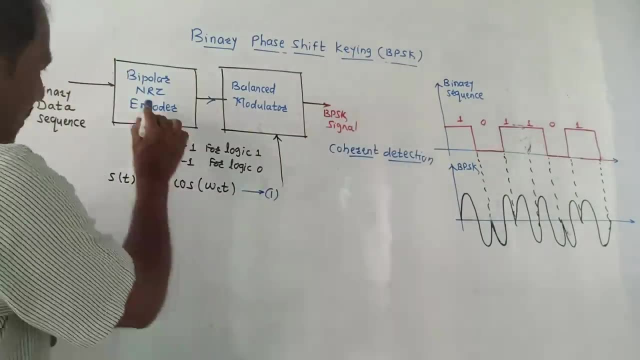 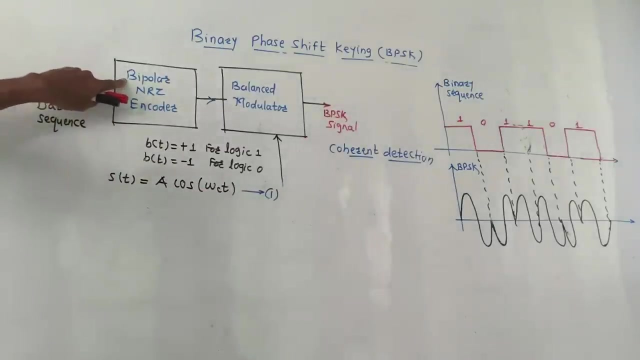 First block is binary NRZ, bipolar, NRZ- encoder. Bipolar means both polarities, Positive as well as negative. NRZ means non-returned to zero. It is one of the format of representing the digital data, So we are using bipolar. 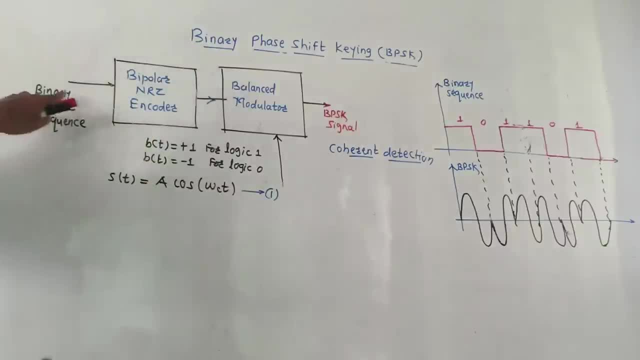 NRZ encoder. Function of this block is to convert the binary data. Binary data means, like I told, logic zero, logic one. It is the data of this form. It is to be converted by this format, By polar NRZ format. The next block is balanced modulator. 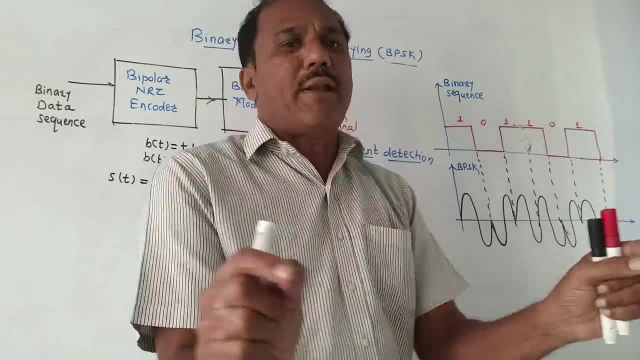 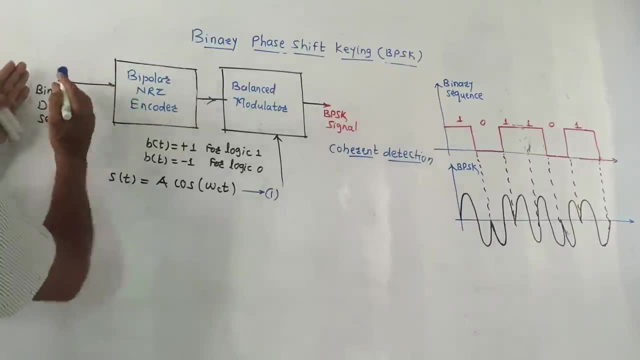 Balanced modulator, in very simplified language, is the multiplier. one input of balanced modulator which is a multiplier modulator. that is the bipolar energy signal, but the binary data was commonly energy had not returned to zero. signal may convert. yeah, that is one of the 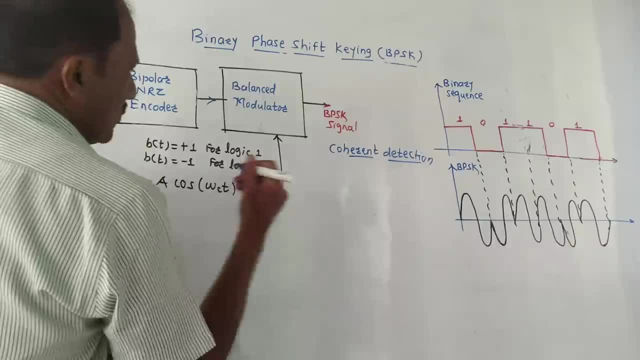 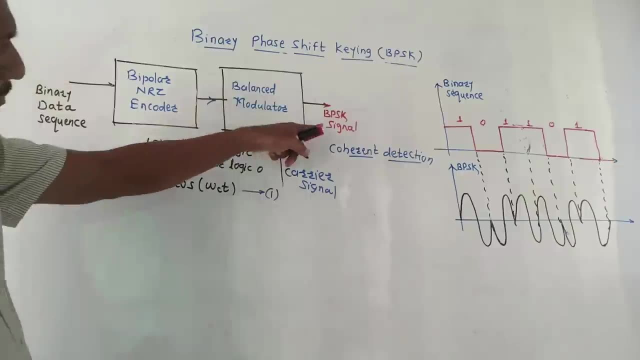 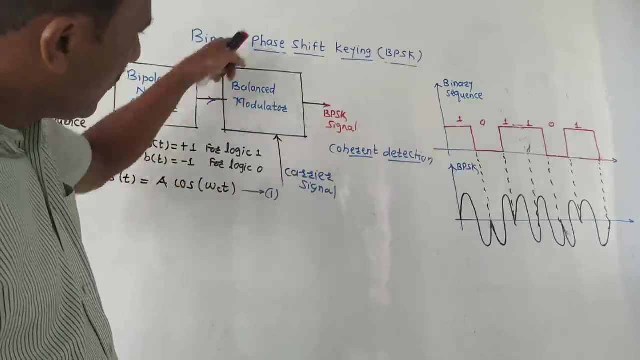 inputs. second input is the carrier signal. so you have a envelope carrier signal applied. then output of this block- that I mean after taking multiplication of this bipolar energy signal and carrier signal, which is done. this multiplication is done by balanced modulator. output is BPSK signal, that is. 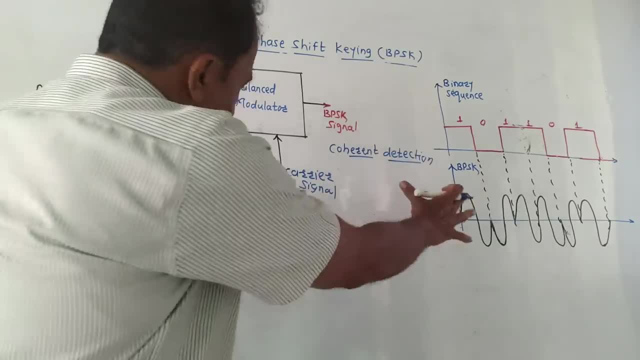 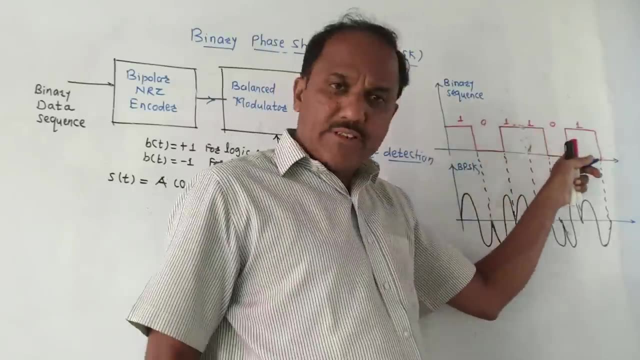 binary phase shift. King signal will discuss the waveform and mathematical part. then this block diagram will be more clear to you. up they go. example: Kilimanjaro sequence, as you can: 1 0, 1, 1, 0, 1. this is the binary data homologo. 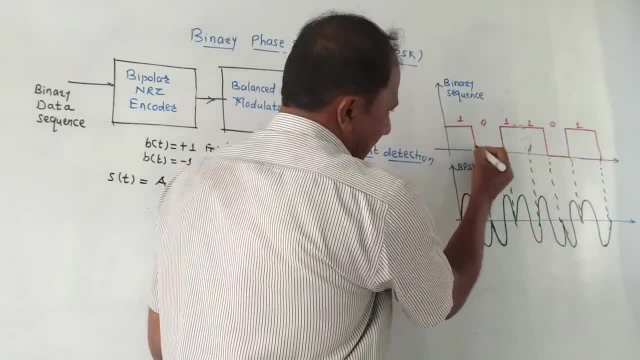 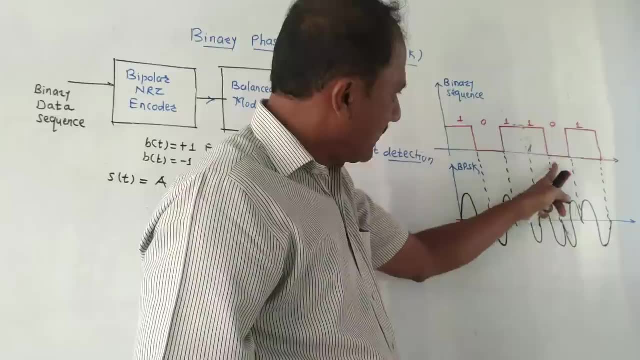 procedure: Patai, how to draw the diagram. your logic one: I do. you have a high decline. logic zero: yeah, we're a zero. they can have. your logic one: hey, again I have shown high pulse. then again logic one, then this is logic zero. and last is: 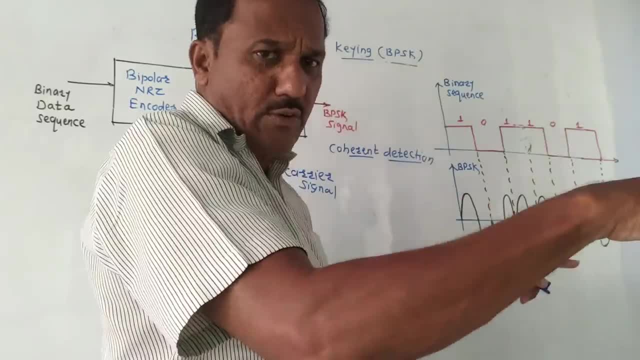 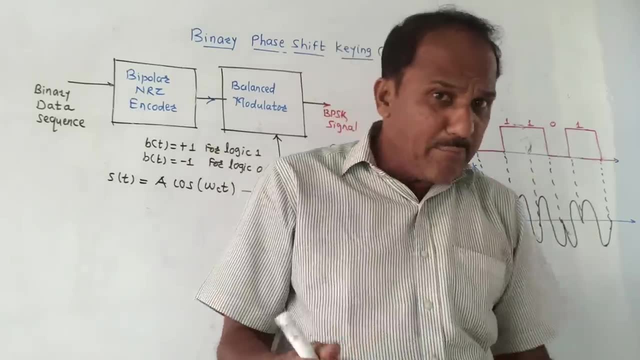 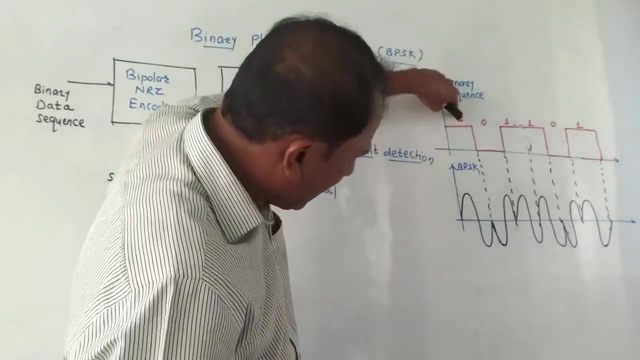 logic one. so logic one killer is a little x square of a man. I have up you just second diagram that is output of for BPSK. yeah, the BPSK, but the phase shift change for a according to the incoming signal. so I say, correlate color logic one head to your part, kill him at the be a hot, see a zero, a baby. 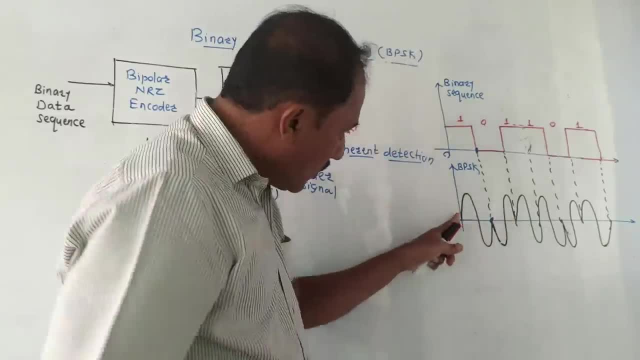 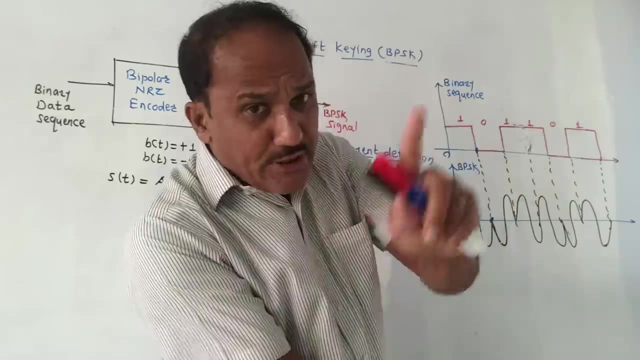 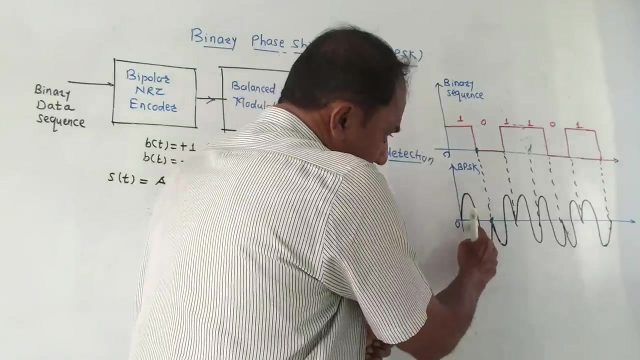 zero a yeah say yeah. logic one hand is parked up, logic one kill a pessoal pickers has action for the 34% of the second half cycle in Japan. activa, BPSK, MCU, have the way hollywood, bpc Lord a ание medicare logic wonder. 25. 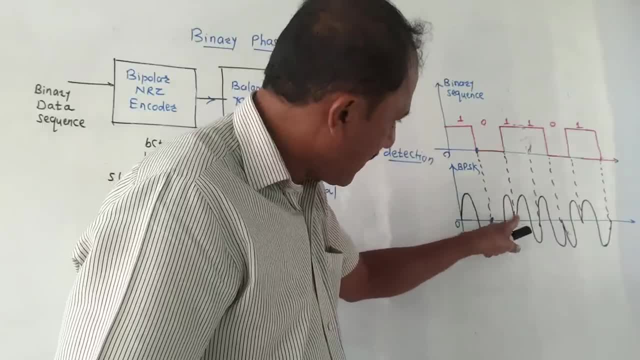 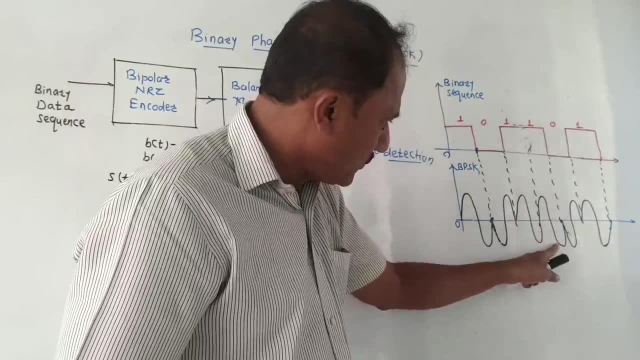 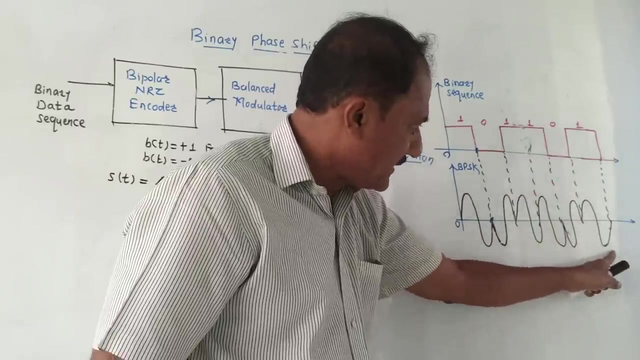 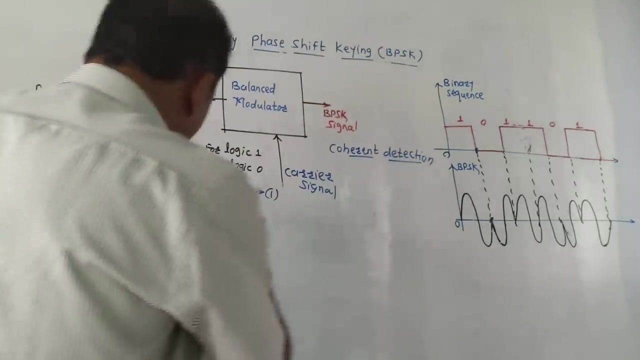 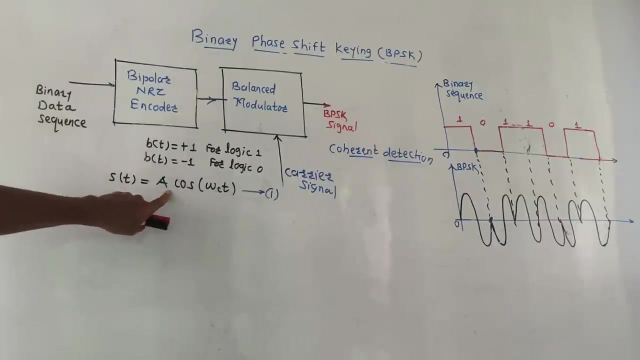 step on the % of 80 kids. Si, okay, then positive. last logic: one, first half part positive, second negative. so this is the waveform related to generation of BPS k signal. now let us talk about the mathematical part. this is the equation of carrier signal. s of T is a cos Omega. 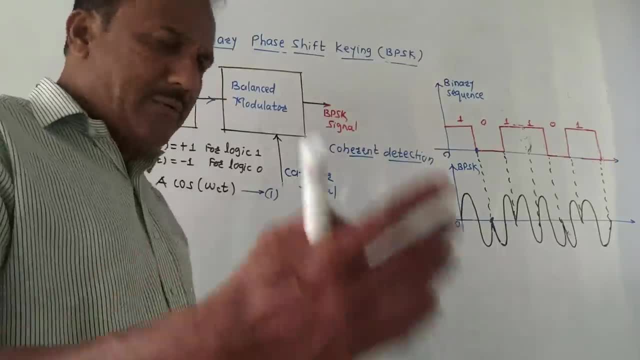 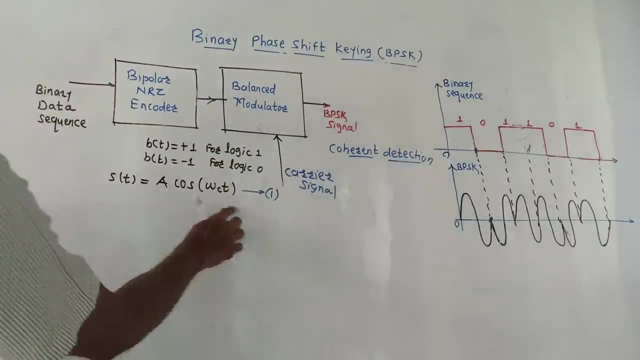 C, T. suffix C stands for carrier is to button up log a B. notation equation. use character a, cos 2, pi, f, 0, T. anything will do so. this is the equation of carrier. signal out our word. recall Carlo Joe last video. maybe I'm going to. 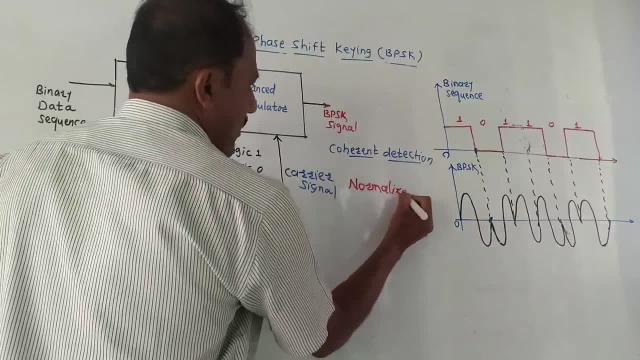 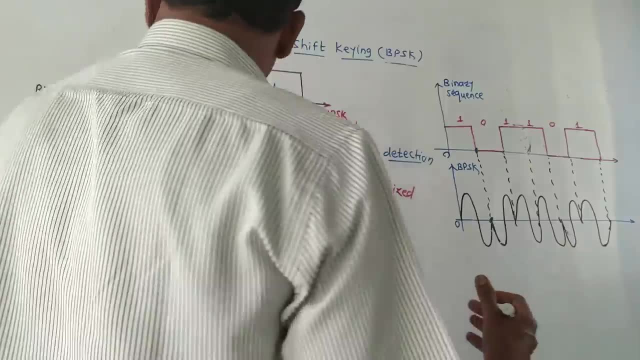 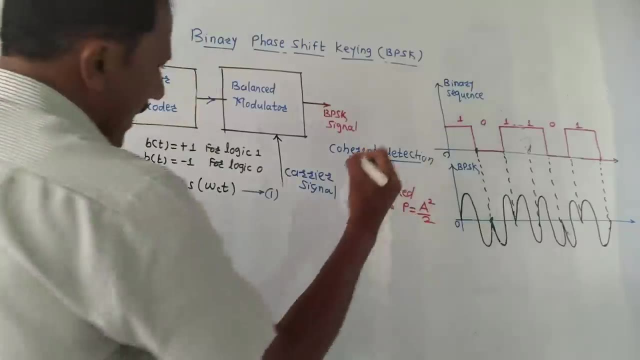 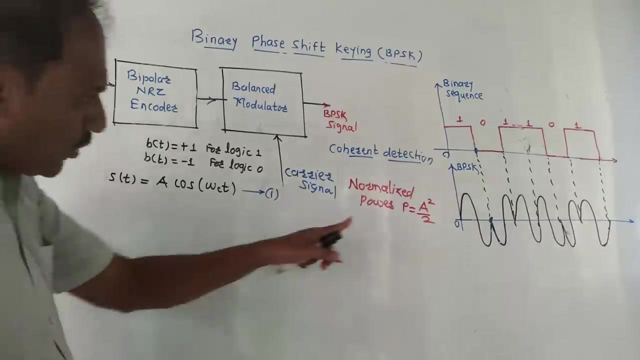 discuss care. it is normalized power. normalized power, basically meaning of word normalized, means value of resistance is one over recall the formula normalized power is given as amplitude square upon 2. amplitude square upon 2. a is the amplitude of signal, amplitude of the carrier signal of the normalized. 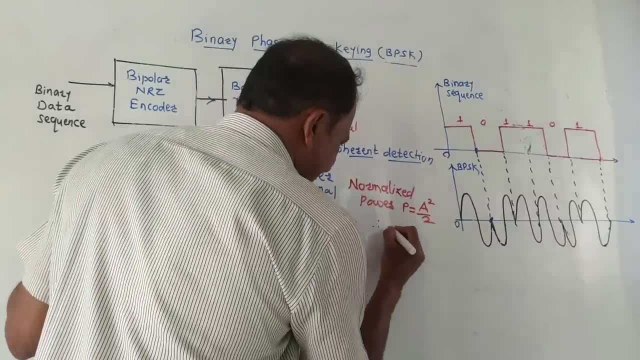 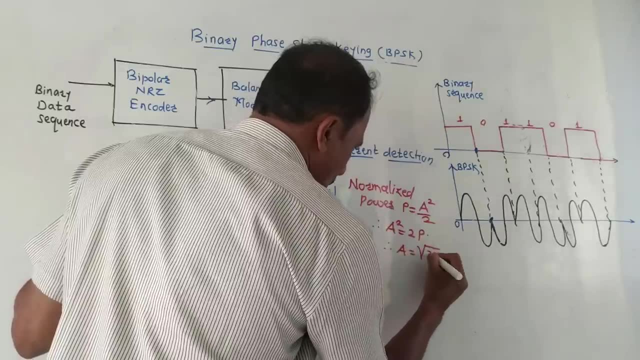 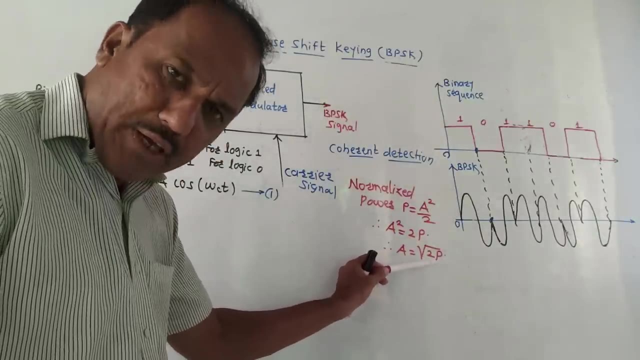 power equation of a square upon 2. so from this I can write: s square is equals to 2 P. therefore a is equals to square root of 2 P. so we have written expression of a in terms of P, where P is the normalized power. so this equation. 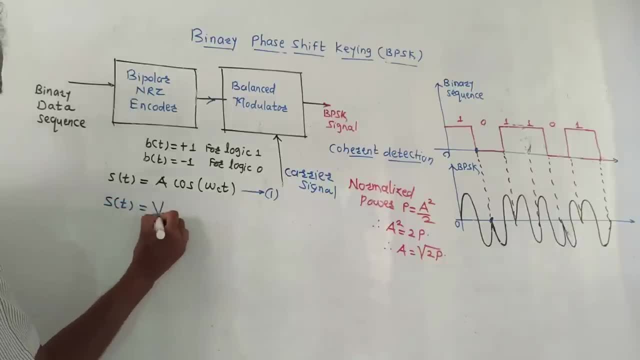 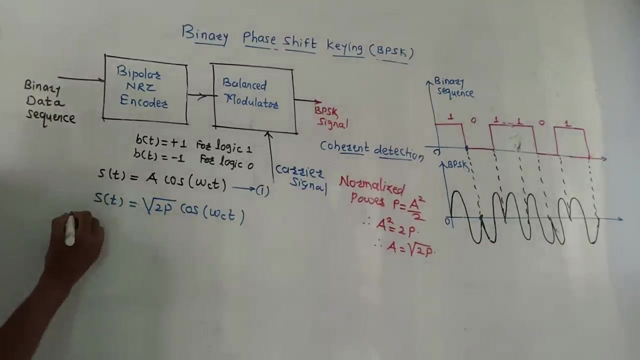 can be written as: s of P is equal to square root of 2 P, cos Omega, C, T. what I did, just a replaced a by square root of 2 P of those symbol of low. consider that a first for logic 1 or for first symbol. same equation can be written as s 1 of P, but logic one, pilot. 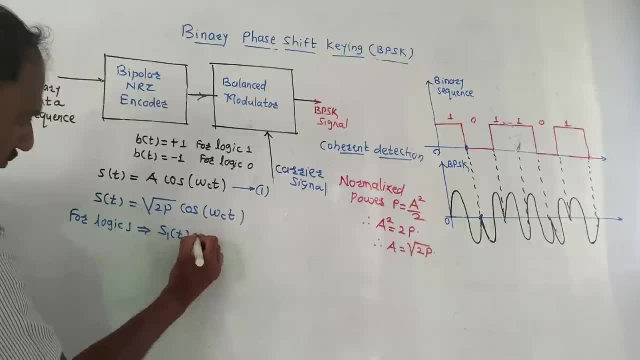 symbolic according to this diagram. so I have denoted it by s 1 of P, which is root 1 of T, root 2p, cos, omega, ct. Then for logic 0,, next symbol, they call logic 0. So for logic 0,. 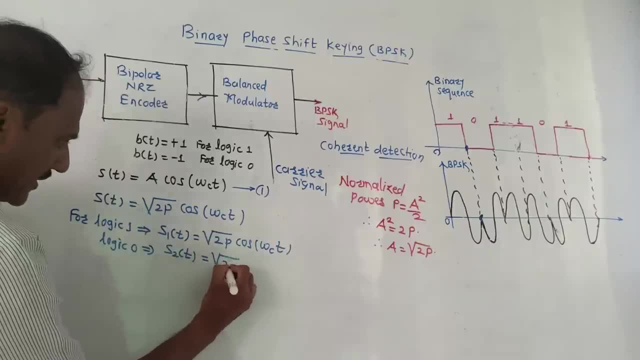 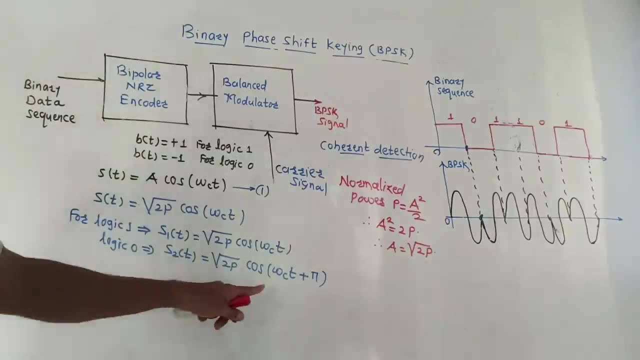 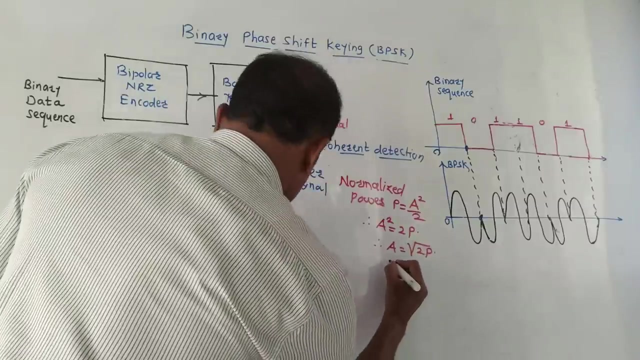 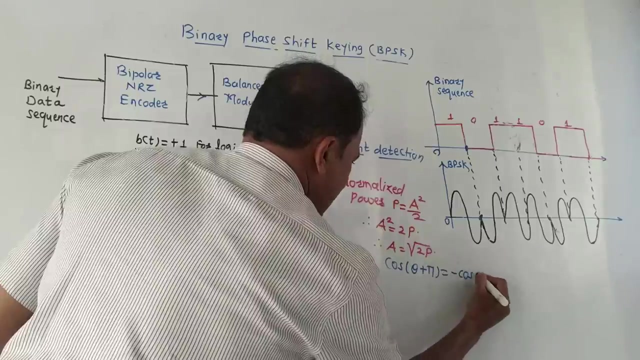 I will denote it by h2 of t, which is same equation, root, 2p, cos, omega, ct plus pi. Why? Because just now we discussed the diagram. There is a phase shift of pi. Now recall the mathematical identity. Mathematical formula is cos. theta plus pi is equals to minus cos. 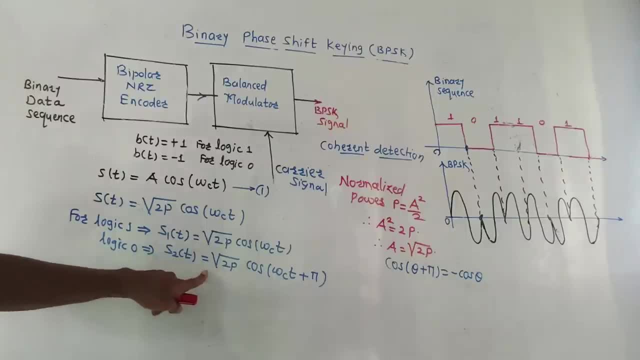 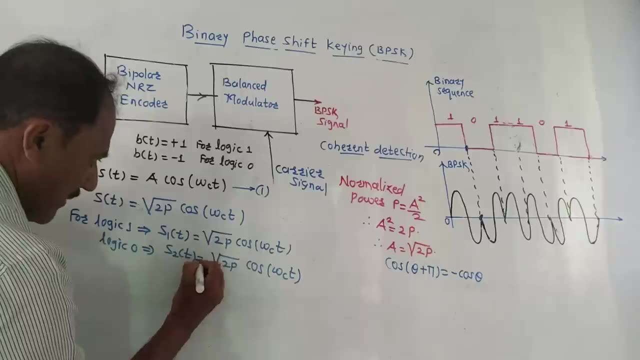 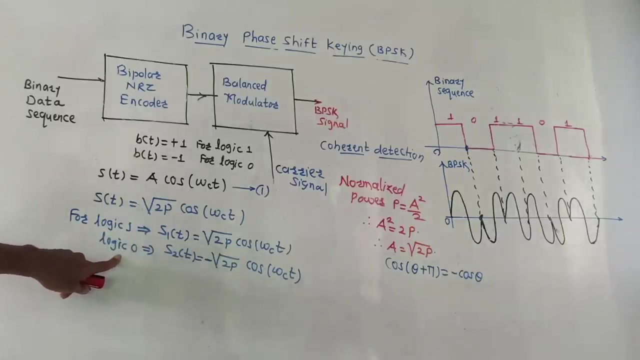 theta. So I will just replace this pi. I mean delete this pi and I will put a minus sign over here. So this is the equation of h2 of t, That is the bit related to logic 0.. So we have written the expression. 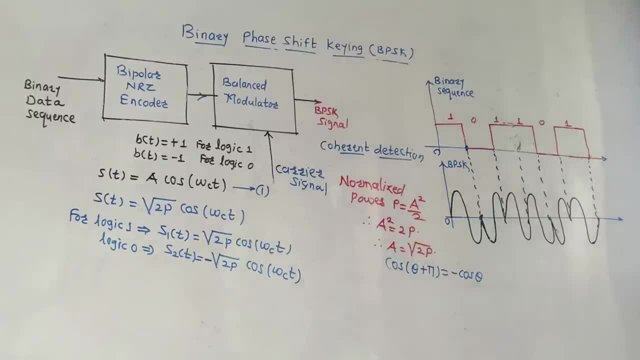 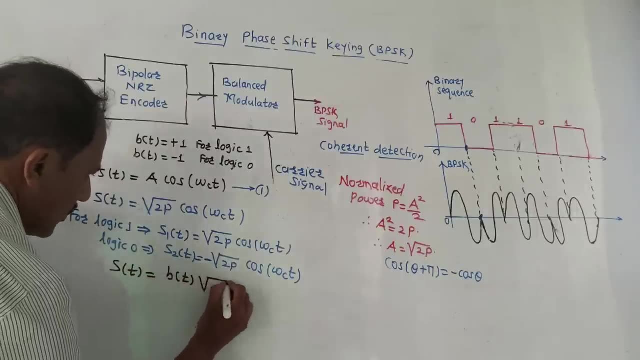 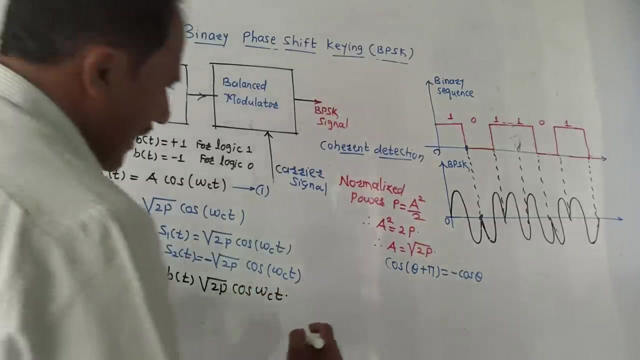 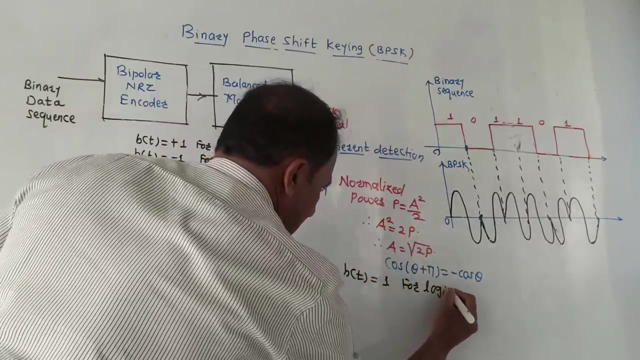 In terms of logic 1 and logic 0.. Now this expression can be written as a generalized expression like this: b of t, root 2p, cos, omega, ct. Here I have used a symbol: b of t. Now how to remember: b of t is equals to plus 1 for logic 1 and b of t is equals to 0 minus. 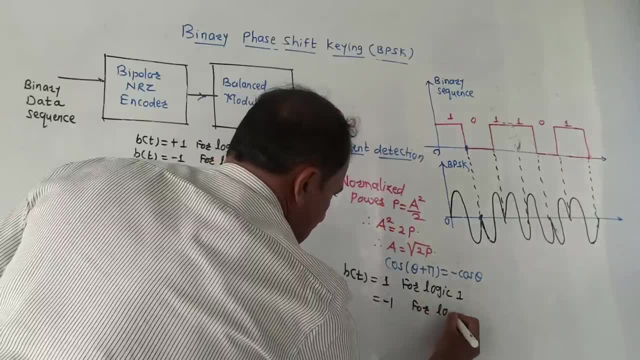 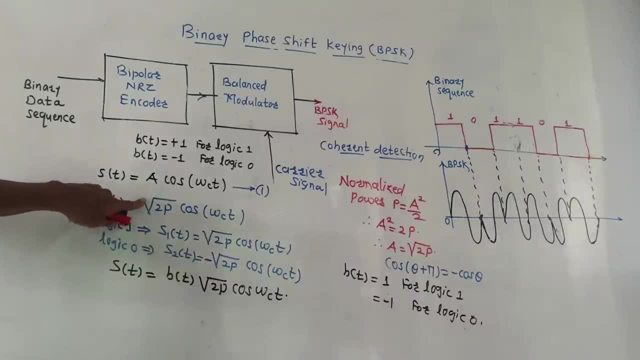 1. b of t is minus 1 for logic 0. So I have absorbed plus and minus sign in this equation, Because here once plus sign will come for logic 1 and for logic 0 minus sign will come. So I have written it in terms of b of t. Now last step: This power. power is denoted by p Energy. 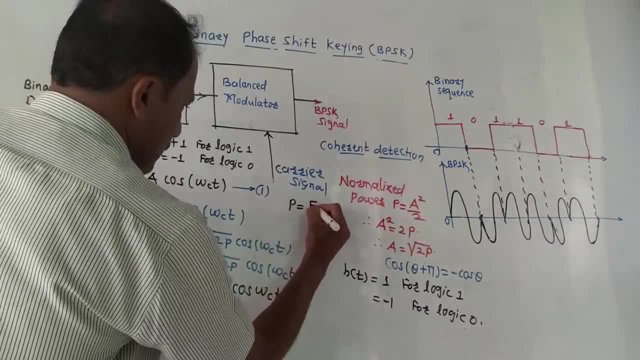 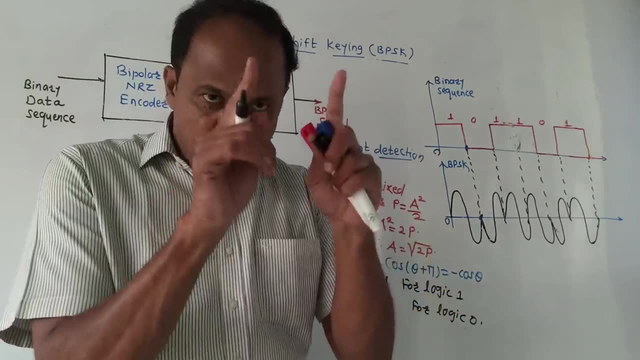 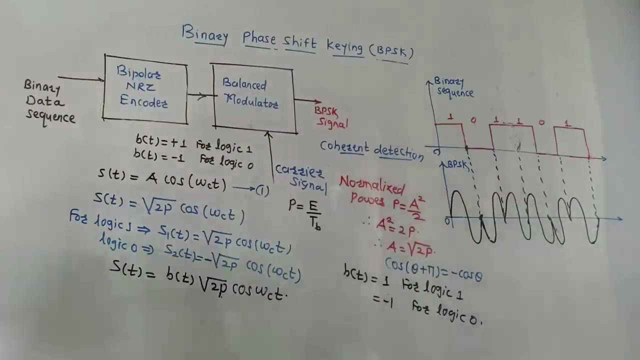 and power are related as p is equals to energy upon time. Here I write tb, That is a, b of t. This is the bit duration. Basic formula is: power is energy divided by time. So power is e upon tb, tb is the bit duration. So I will write the equation of BPSK signal like: 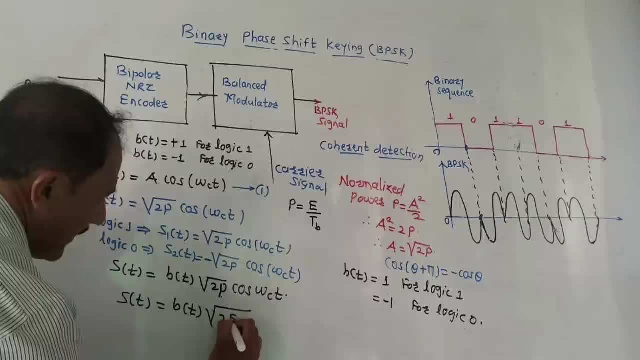 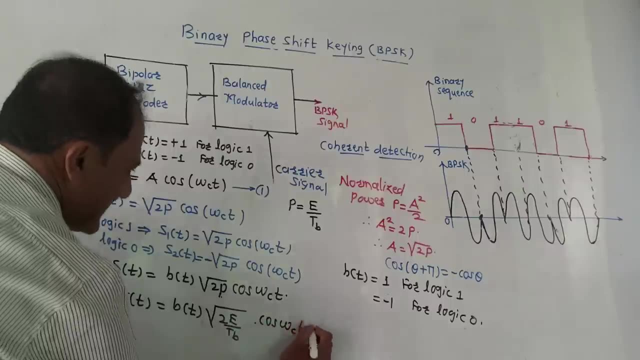 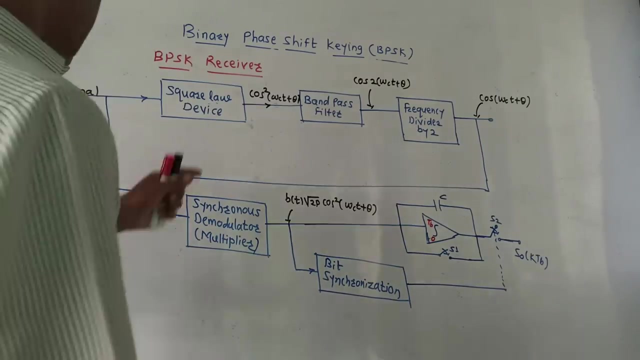 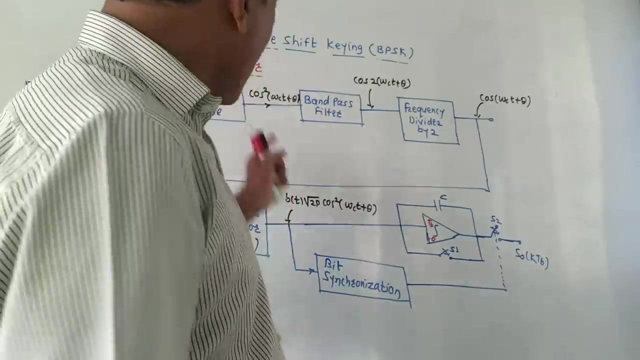 this Square root of 2 e upon tb. Same equation cos omega ct. This is the equation of BPSK signal. Next is the block diagram for BPSK receiver. as I told you in exam point of use, a separate question can also be asked to draw and explain the BPSK receiver. 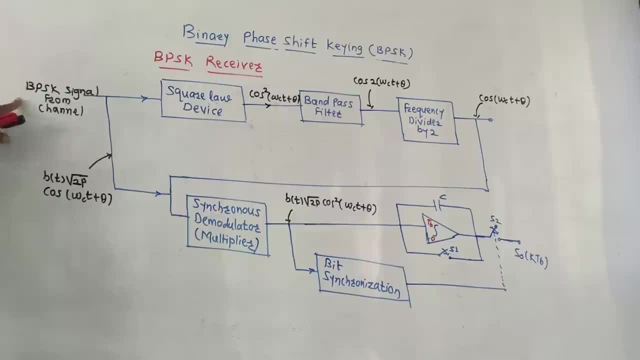 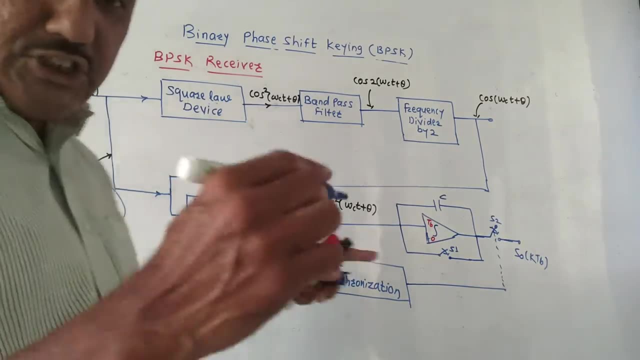 So this is the block diagram of BPSK receiver. Here see BPSK signal. from the channel which is having this equation just now, we have derived this expression. This is the generated BPSK signal. This is the block diagram of the receiver. 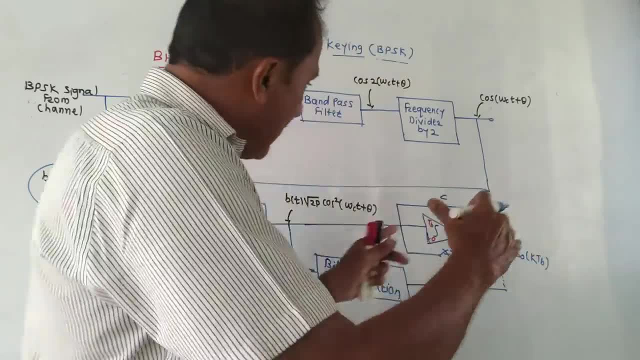 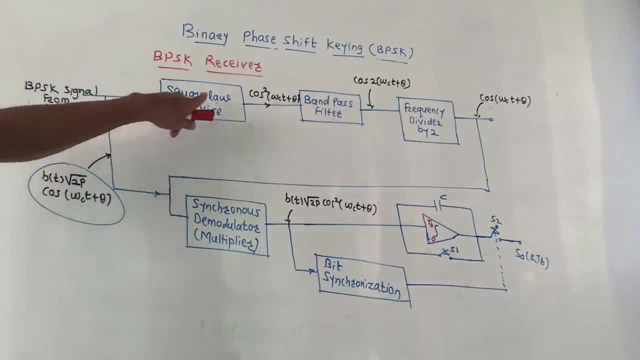 Now see, I am going to do the mathematical analysis. first I will explain this block diagram. after that we will do the mathematical analysis. So first block is square law device. as the name indicates, it is taking square of the incoming signal. 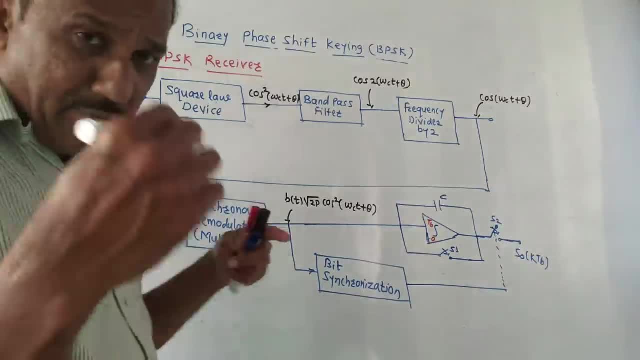 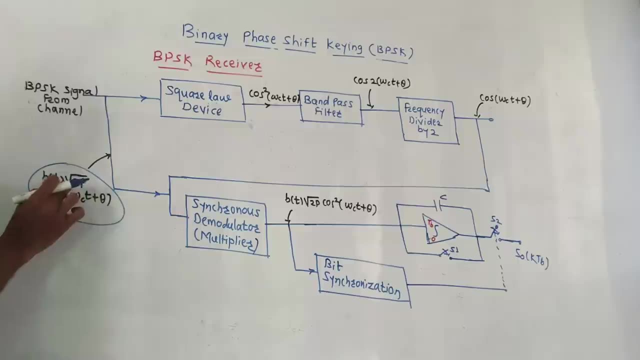 Incoming signal means we are not interested in magnitude of signal, we are interested in phase shift. That is why, after taking square it will actually come Bt square and this square root will vanish. but I am skipping the magnitude, Just for simplicity. so this same signal is applied here also. the output of square. 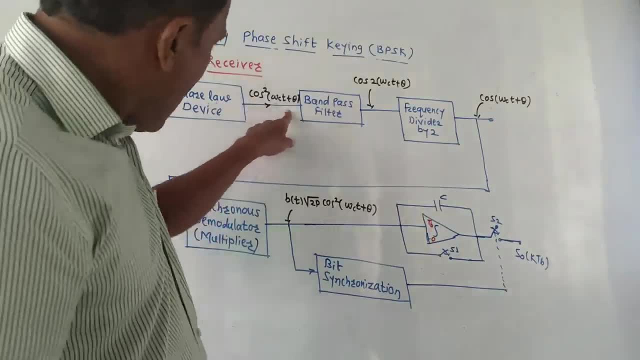 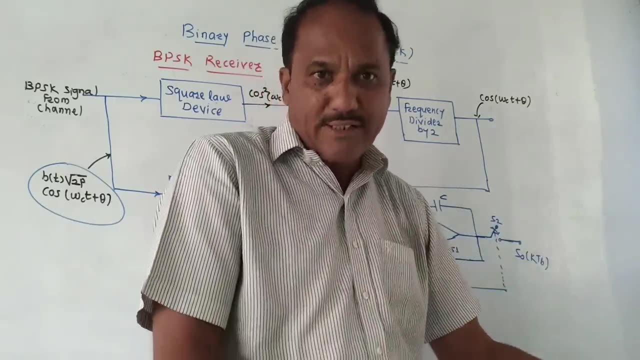 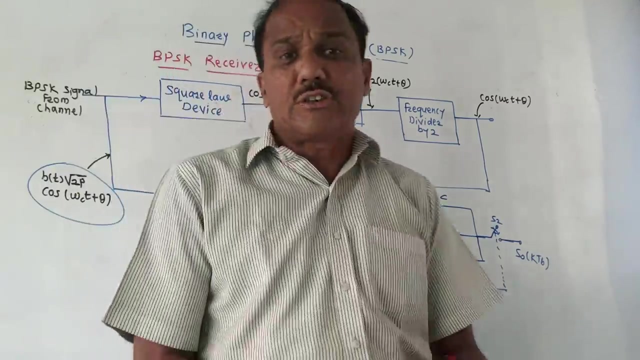 law device will come cos square, omega, ct plus theta. now, this term of cos square, we have to make use of mathematical identity. we will cover this in mathematical analysis. So, presently, cos square, which term is coming? omega, ct plus theta? why this theta is introduced? 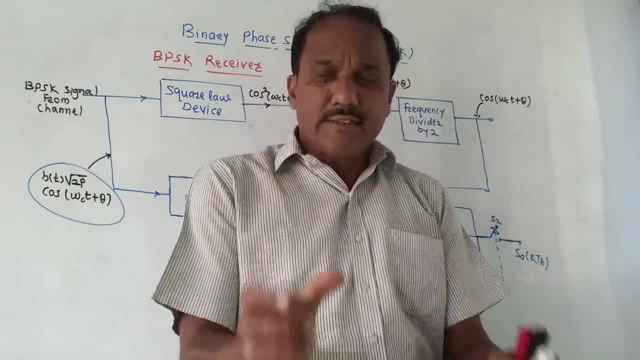 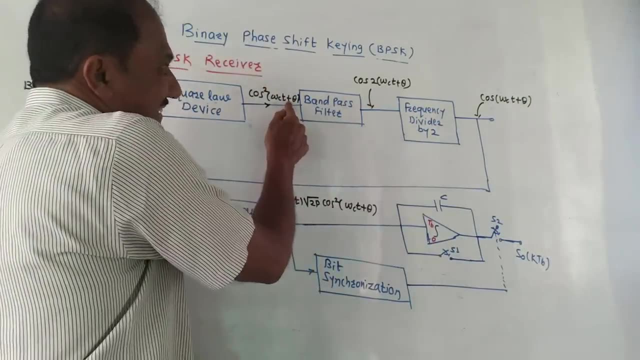 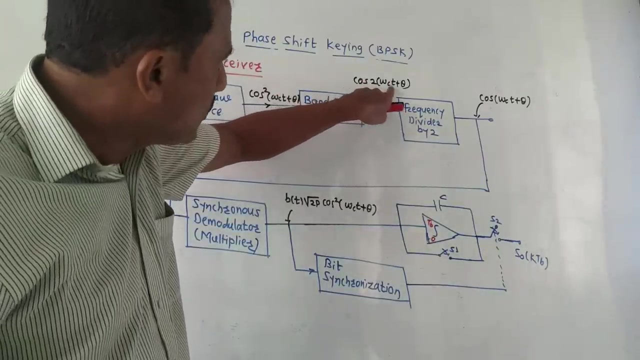 theta is basically phase difference or delay, as you see, to get signal from the transmitter to the receiver. That time period is denoted by this term theta. now we will do this mathematical calculation. we will convert cos square like this: so it becomes cos 2, omega, ct plus theta. it is passed. 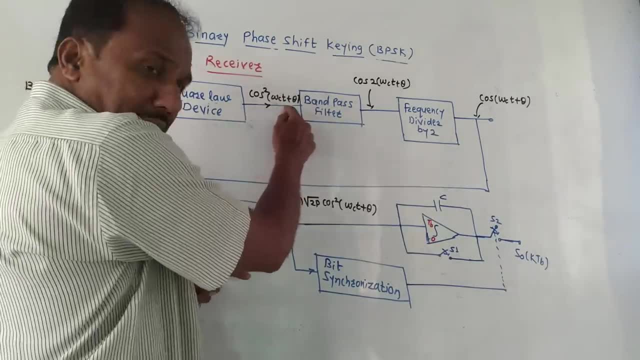 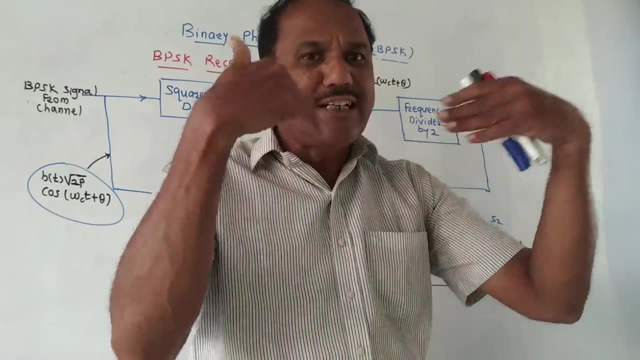 through the band pass filter. now see, we will convert this to mathematical part. then it will be passed through the band pass filter. the function of band pass filter is to remove the DC component, or constant term. after that this output will come cos 2, omega, ct, plus. 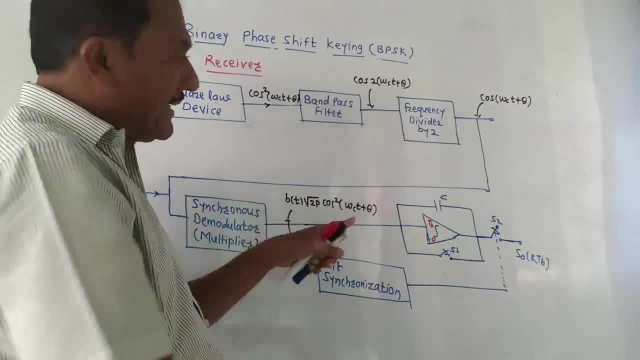 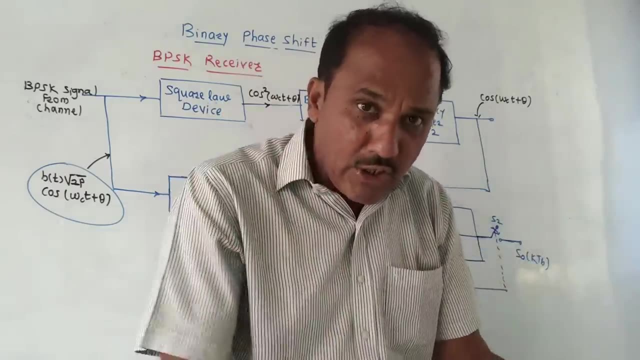 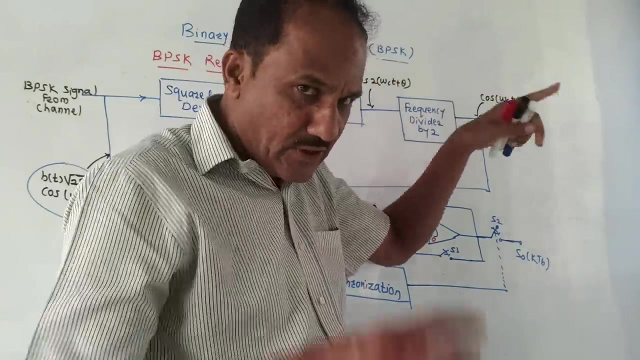 theta again. I will explain this in the mathematical part. this is 2 times value, 2 times omega ct. that means the frequency, carrier frequency is getting doubled. so to recover it, frequency divided by 2, means this: 2 into omega c is coming. omega c is the carrier frequency. 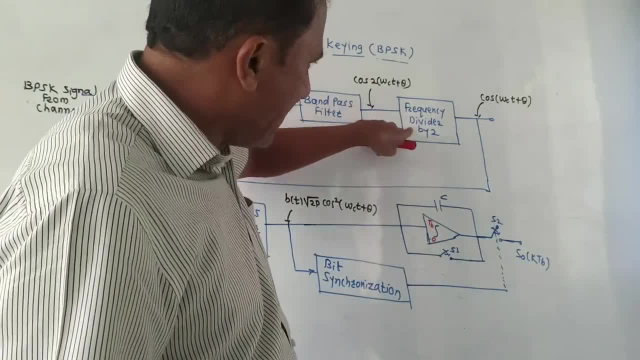 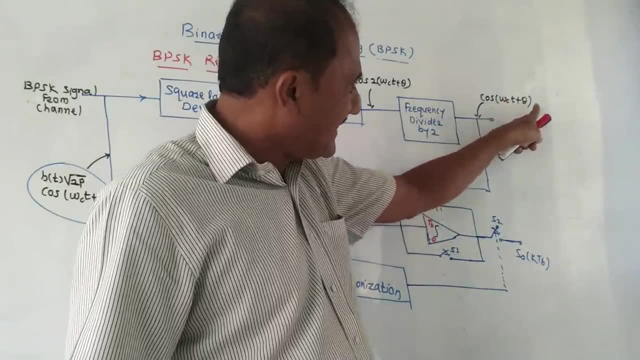 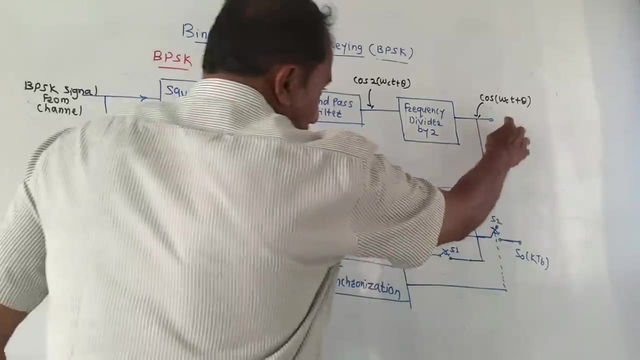 to obtain the original frequency we are using frequency divider by 2, so at the output of this frequency divider by 2 circuit block we are getting cos, omega, ct plus theta. then this signal is applied to synchronous demodulator or multiplier. so one input to this multiplier. 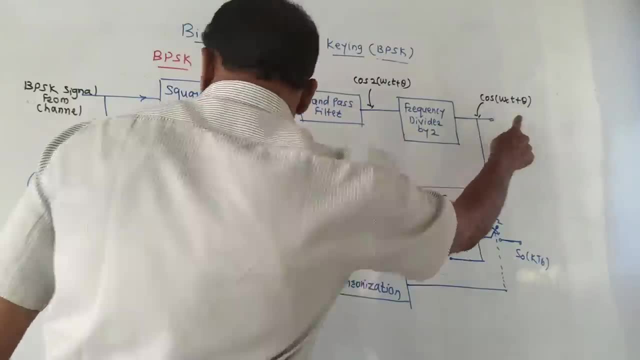 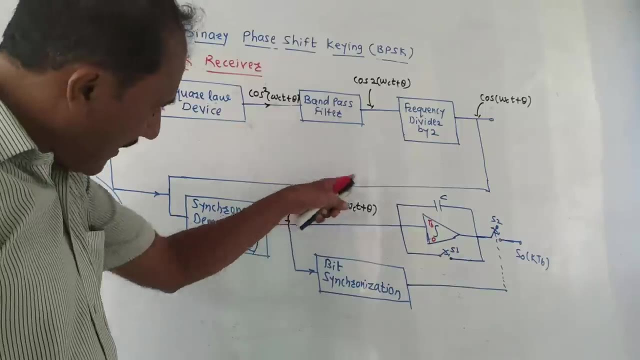 or synchronous demodulator, is cos, omega, ct plus theta carrier signal. second, is this signal which is coming from the transmitter side. so this is the equation of the output. again I will cover this how this equation is obtained in mathematical analysis bit. 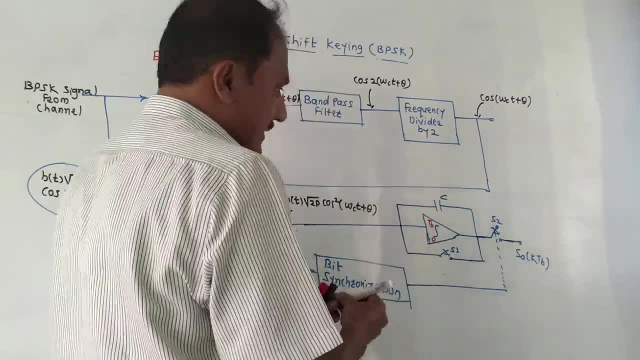 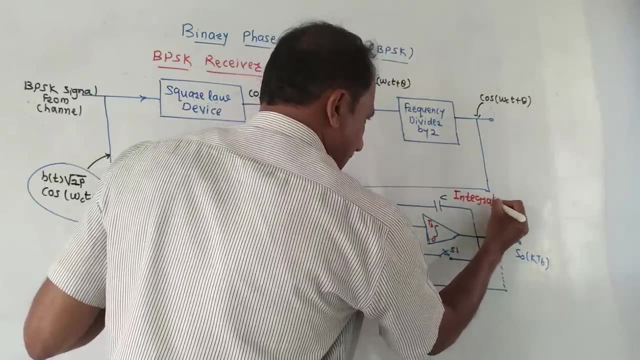 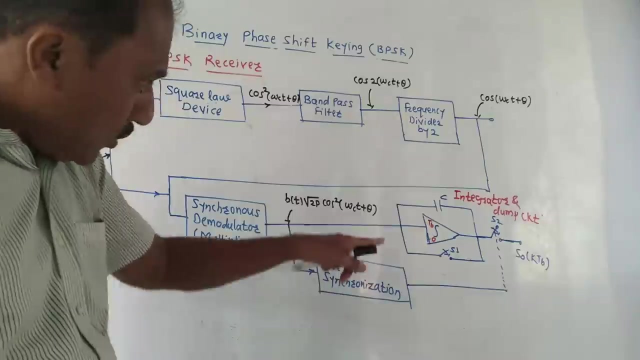 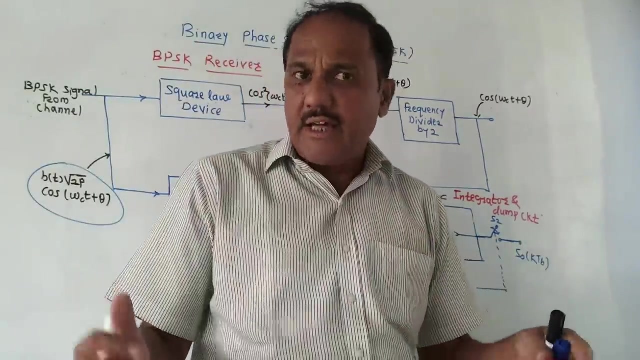 synchronization. see, this is the part. This is. We learned this in the last session. this is integrator and dump circuit. we have well discussed this circuit in the earlier session. so yes, is my integrator. use correct integrator delay, they go home. local signal integrate kernel only. 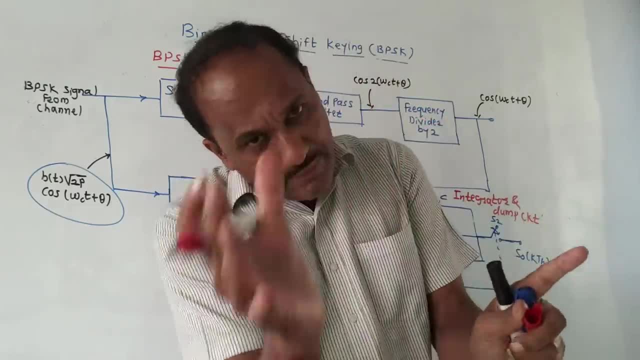 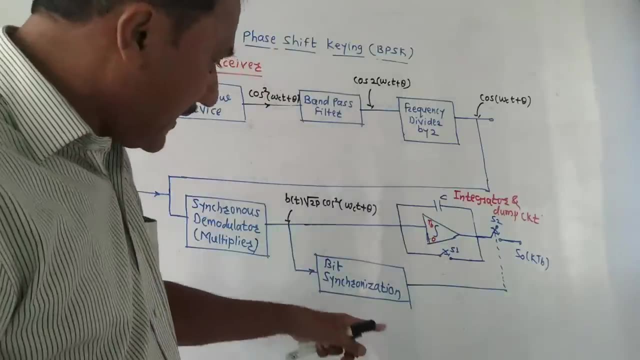 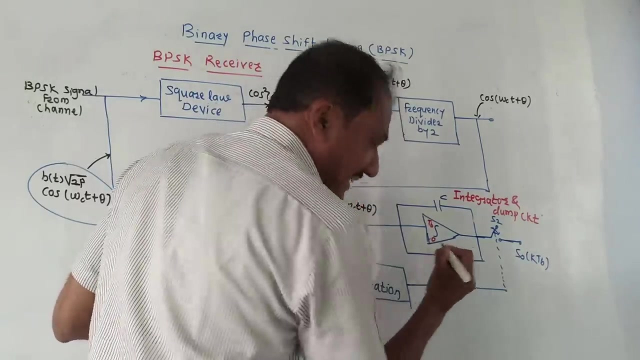 for one bit duration with a 8-bit just time period killer. hey say it is from 0 to TB. TB is the bit duration. oh shit, I'm particularly integration karma. so to achieve this, this bit bit synchronization block is used up. Joe s one switch, a yes, which, this is s one switch. pilot, a current, a her egg bit. 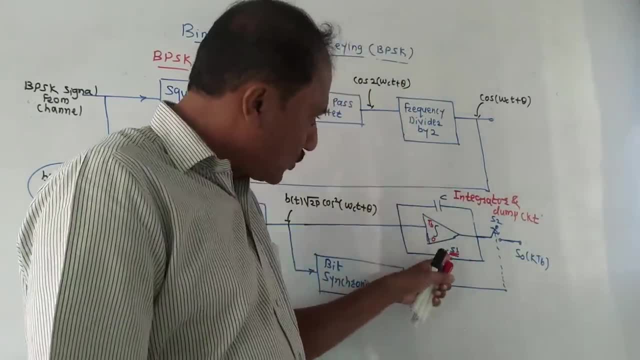 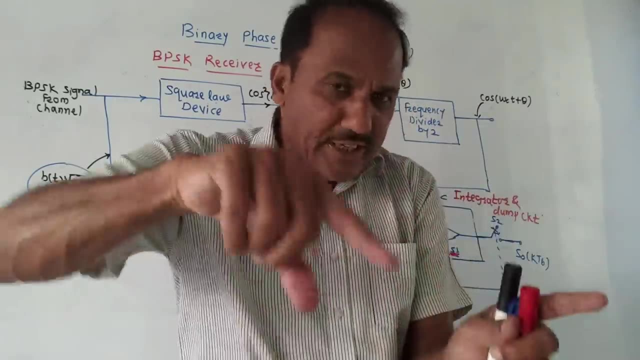 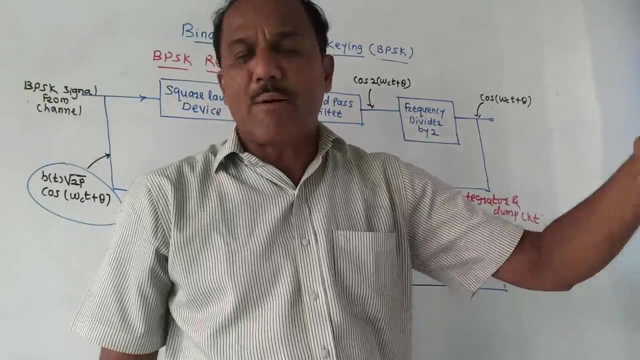 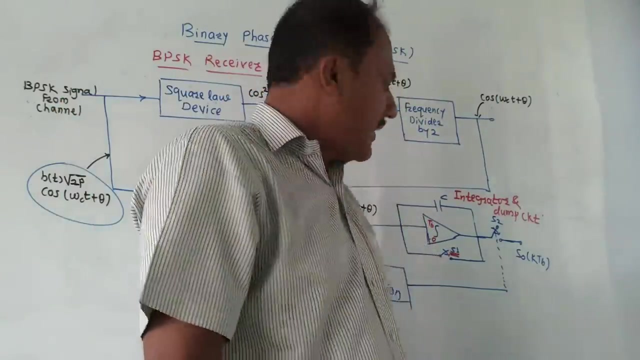 Kelly, a first s1 switch is closed so that capacitor will be fully discharged and then whatever incoming bit is there for that bit, integration is performed from 0 to TB switch, a s 2, that is output switch or sampling switch, her egg integration, complete or a kebab. this switch is closed and the sampled value is made. 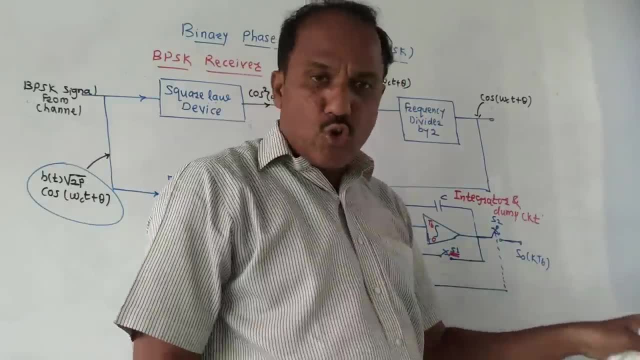 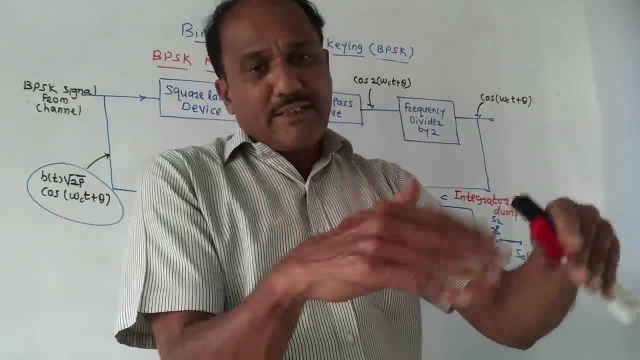 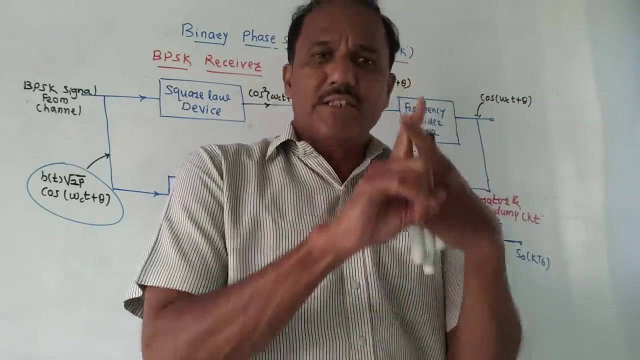 available at the output. so output is denoted by a 0 k TB escape bad egg decision circuit use current. yet the function of decision circuit is by considering probability of error and all that the function of decision circuit is take a decision whether the received signal is logic one. 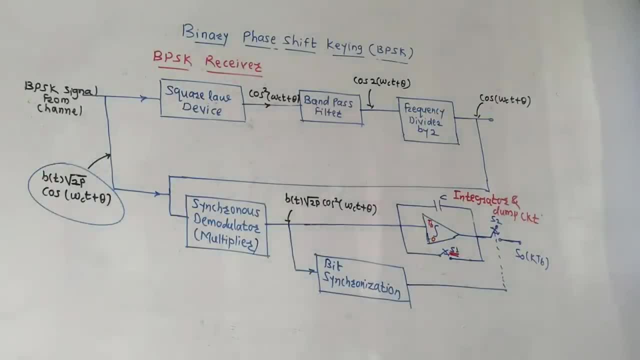 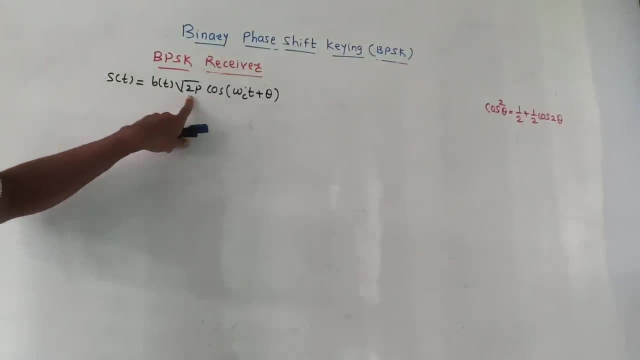 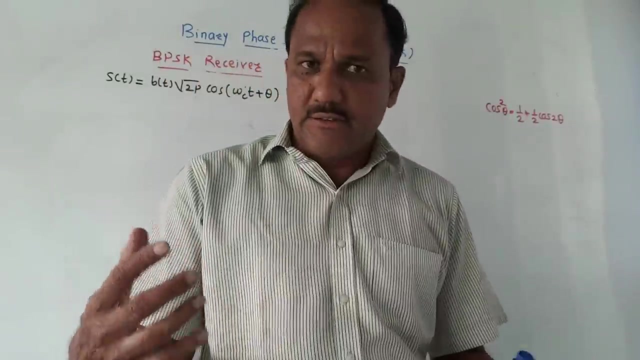 or logic 0. now let us perform the mathematical part related to this. now the equation of received signal at the receiver is a softy is B of T into root 2, P, cos, Omega C, T plus theta. up come lower. already our transmitter sessions may discuss care. yeah, I think that any other a simple equation of a. why this? 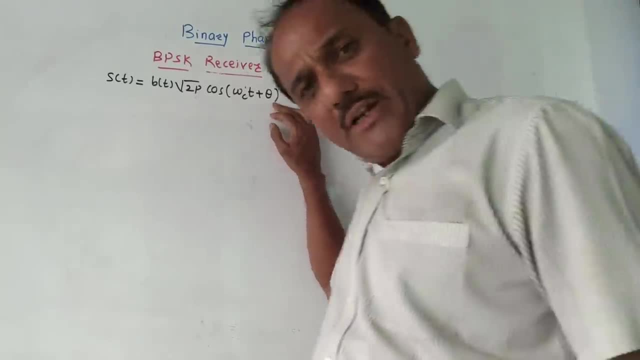 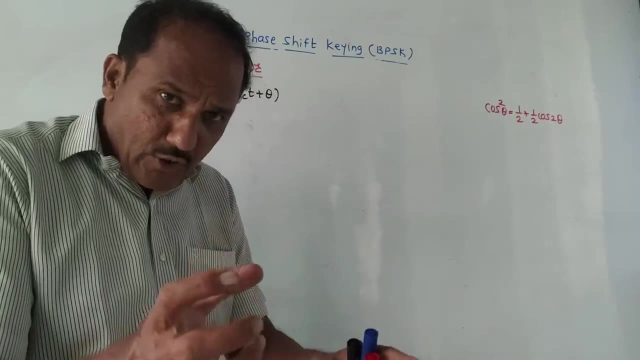 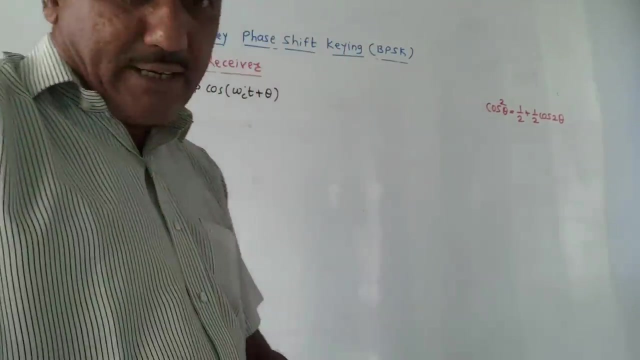 theta is appearing in this equation. just now I explained you, while explaining the block diagram, that the receiver some time period is required to get the signal, but the transmitter signal transmit, cut the receiver to punch link in a touchdown period. look at that temperate. let that time period is called a delay and it is indicated, do not it by theta term of. 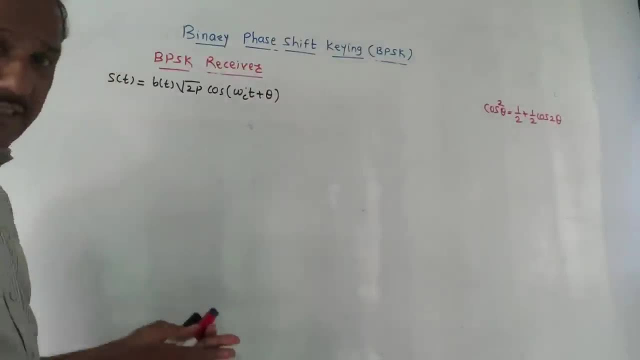 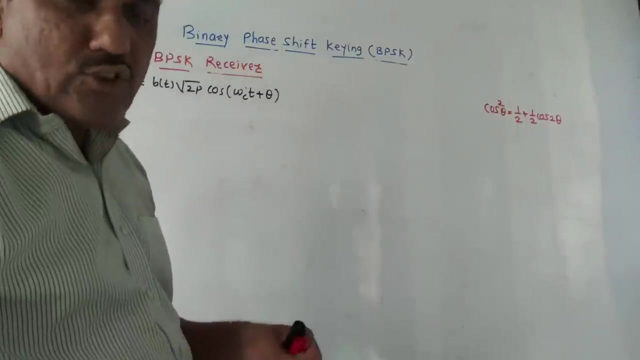 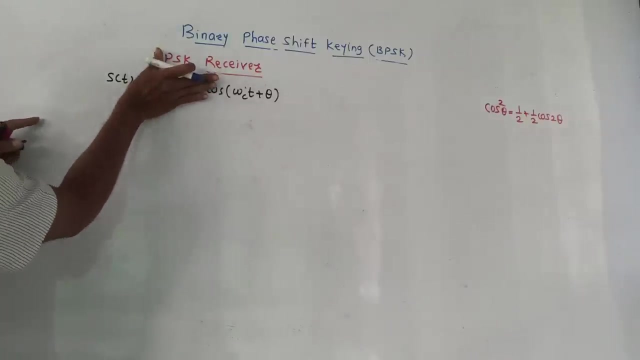 the equal block diagram. prefer call. we are just discussing the mathematical part we already discussed. the block diagram was came up, yet this signal is applied to the squaring device, squirro device. but we are skipping amplitude just for the simplicity. we are not interested in amplitude. 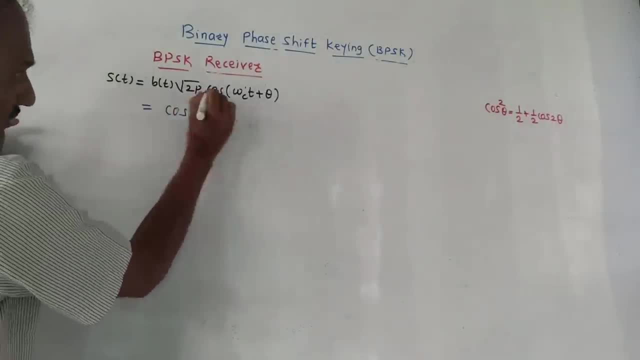 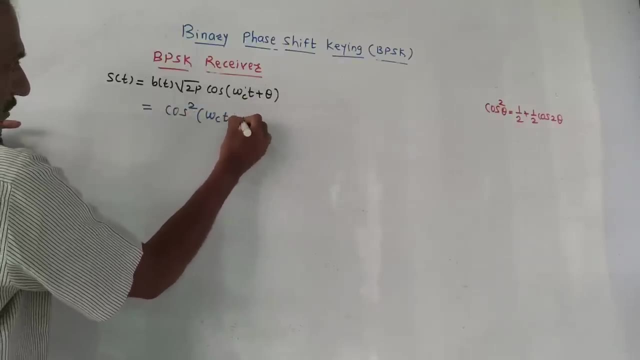 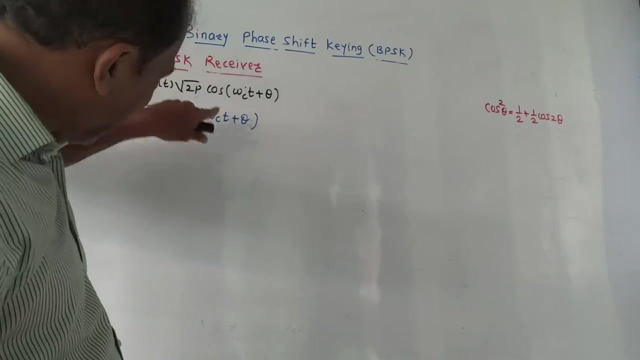 so this same equation. as I told you, I am skipping amplitude, only considering cos term. so it becomes cos square, omega, ct plus theta. now this is the output of square law device. means this incoming signal is applied to the square law device. its function is to take square 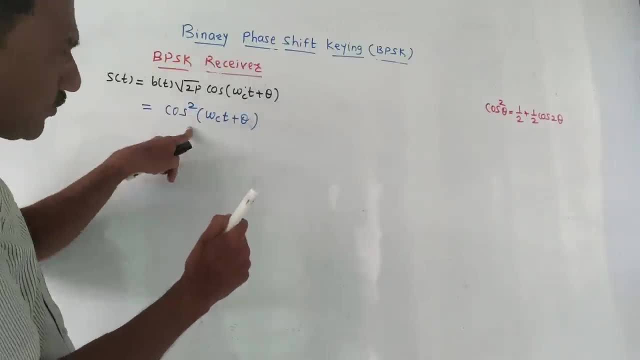 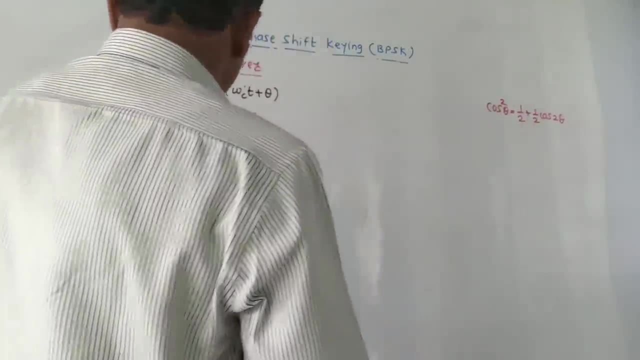 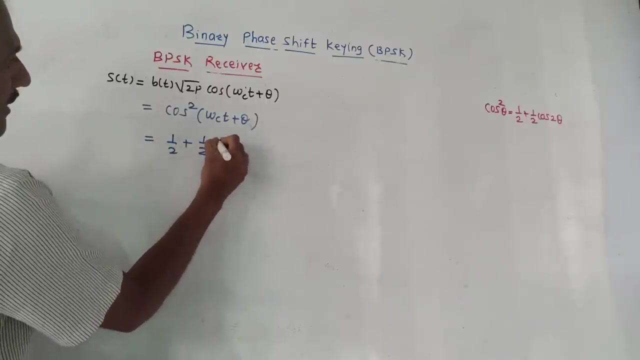 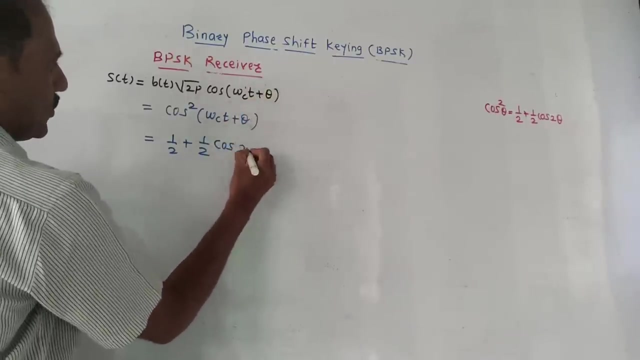 which I have not considered. so this becomes cos square and we have to make use of mathematical identity. cos square theta is one half plus one half, cos 2 theta, so I can write this as one half plus one half cos. I am writing it like this: cos 2 times omega ct plus theta. 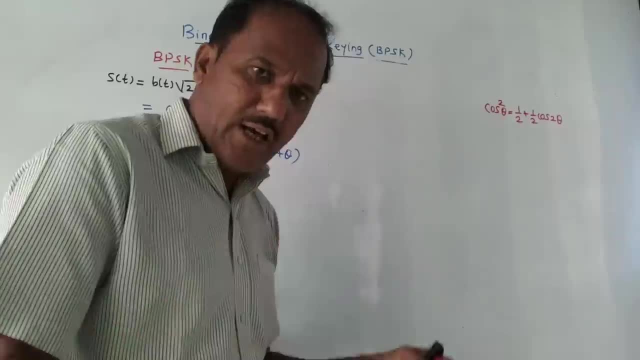 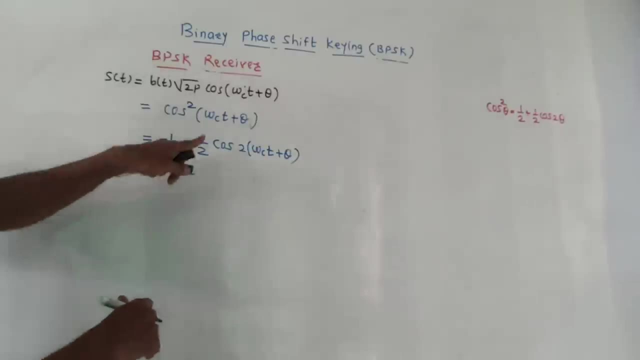 because we have the identity cos square? theta is equal to one half, theta is one half plus one half cost to theta, Don't get confused. So it is one half plus one half this term Now. this signal is then passed through the. 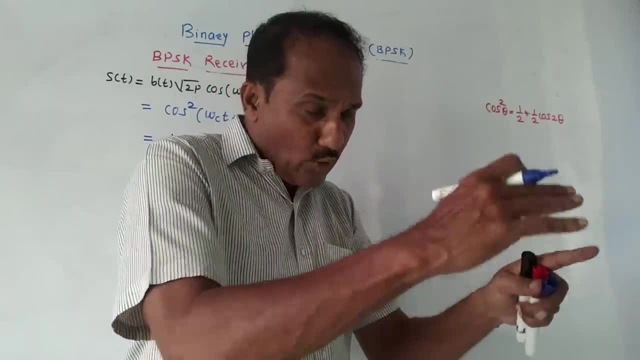 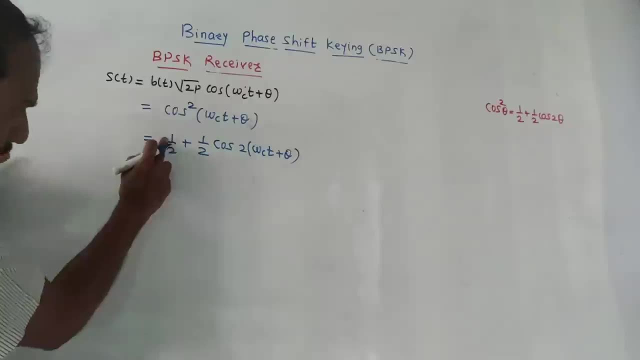 band pass filter. Function of band pass filter- Related Function of band pass filter- is to remove the DC component, DC component. So after passing the signal through brand pass filter, this one half will get cancelled and remaining will be this equation. This is the 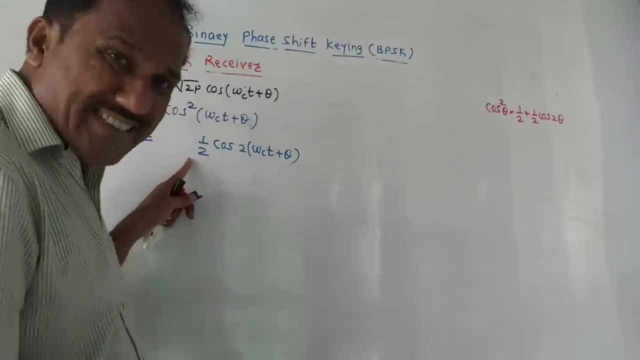 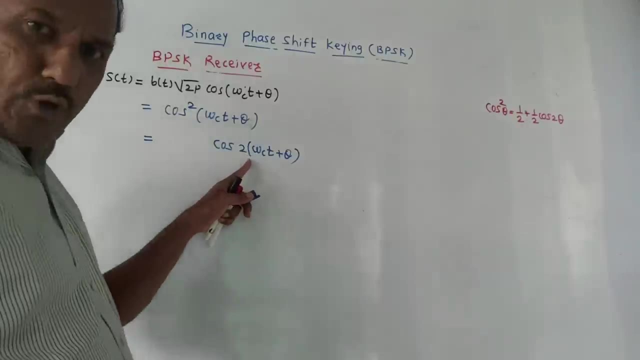 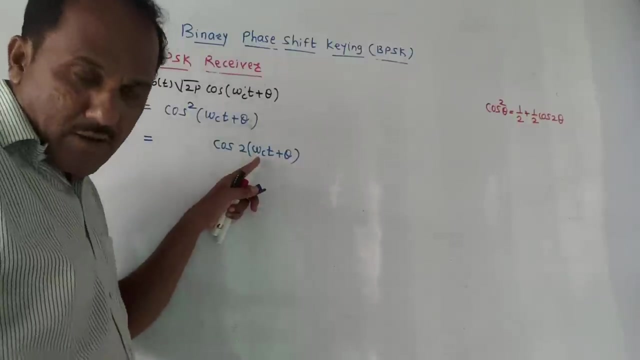 output of band pass filter. Again, this is the one half which is amplitude of this cosine wave. So we are not interested in amplitude, So I am removing this. So this is the output of band pass filter. Here 2 into this term is coming. Ideally it is 2 into omega c. 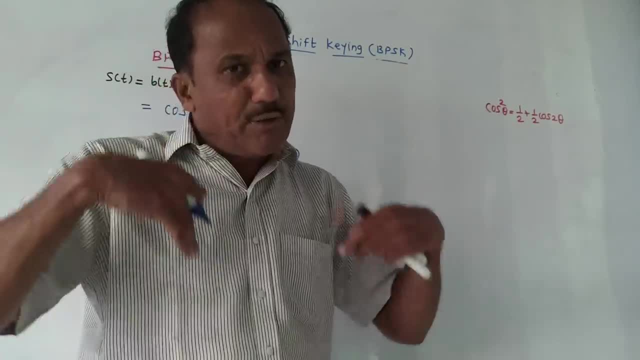 Omega c is the carrier frequency, So the carrier frequency is getting doubled. This is the output of band pass filter. So this is the output of band pass filter. So this is the output of band pass filter. Below this: by this, one half is 1 into omega c. 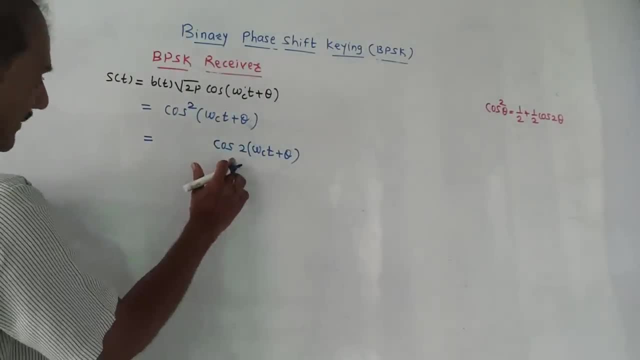 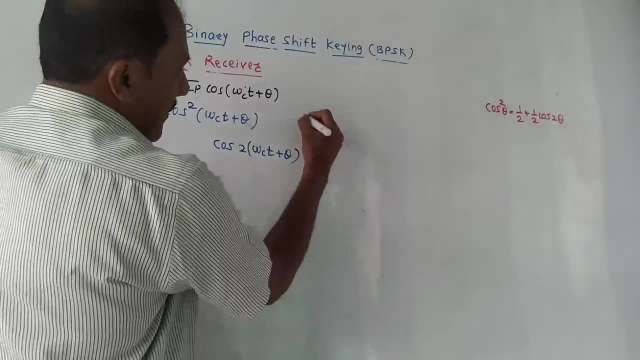 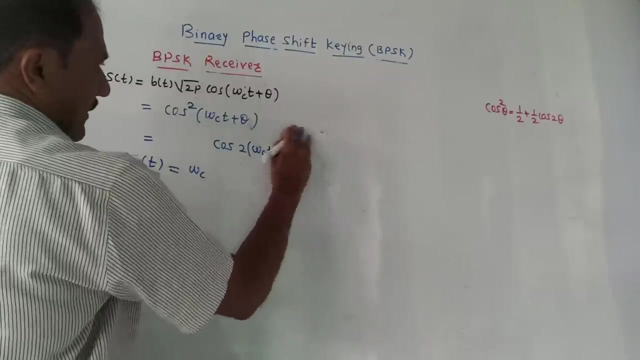 So that means if output of frequency of B now it will be one half growth and so out of this it will go down From here also Output of frequency of omega c. here at this time of the block diagram we have connected it. 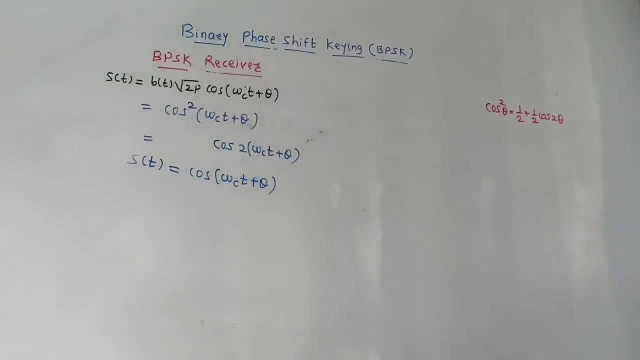 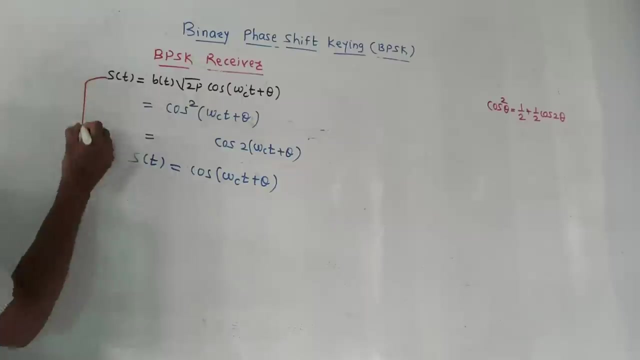 to the frequency divider by 2 circuits. So let's see how this will happen here, plus theta. now refer the block diagram once again. now this signal and the original signal. yeh, yeh, wala, this signal. this, both signal, are applied to the 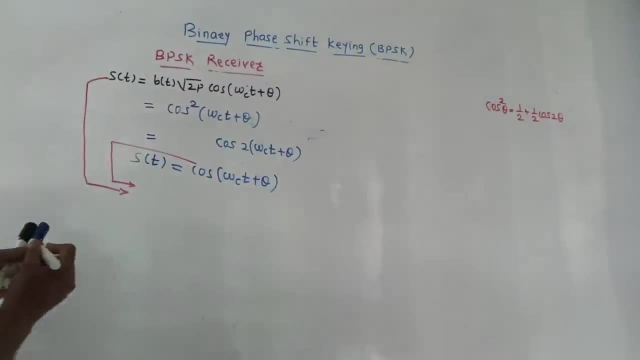 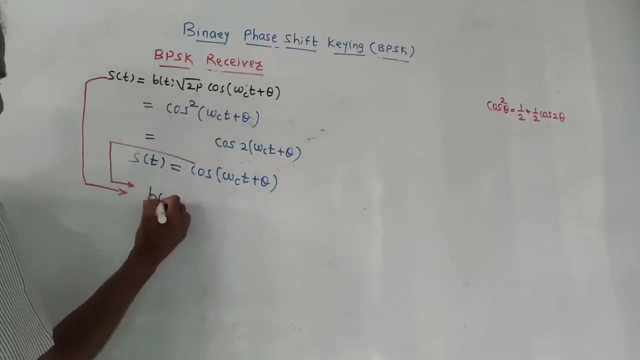 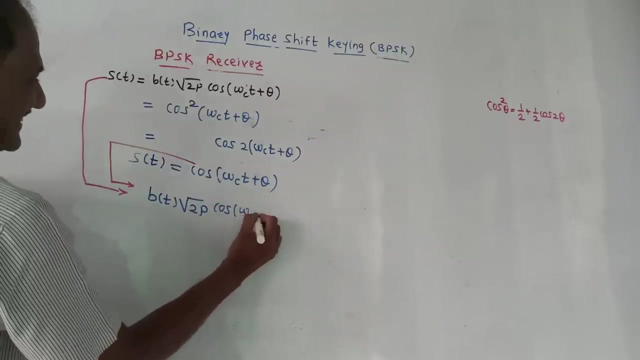 balanced demodulator or multiplier. so output of balanced demodulator or multiplier is multiplication of these two signals. to may yeh yahape aise lagtao B of T, root 2 P into cos, Omega C, T plus theta into cos, into this term cause. 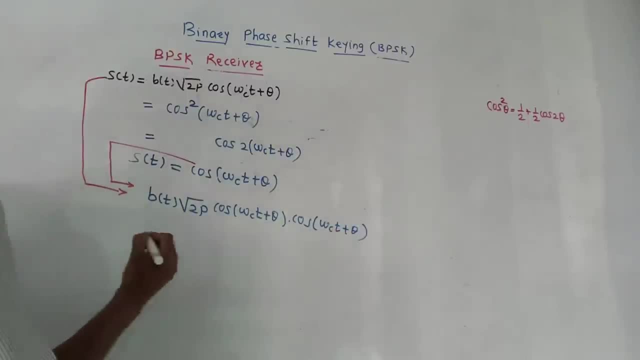 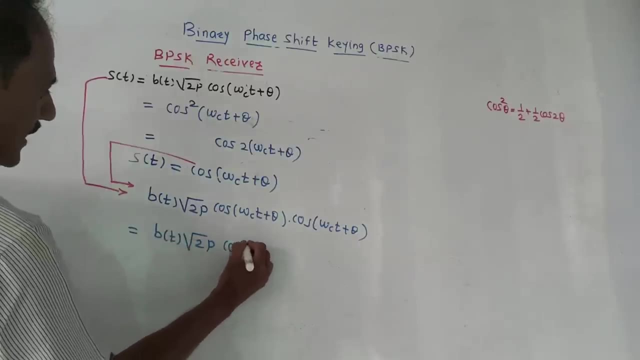 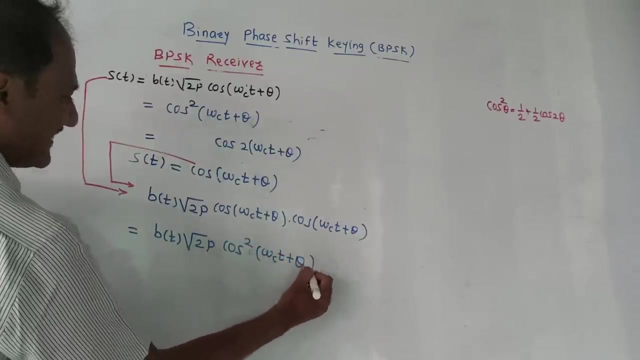 Omega C, T plus theta. so this equation can be written as: B of T root 2, P cos square. this cost into cost becomes cos square for square Omega C, T plus theta, theta. again we have to make use of the mathematical identity: cos square theta is one half plus one. 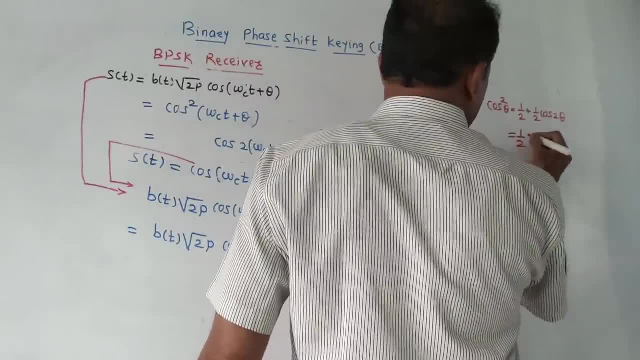 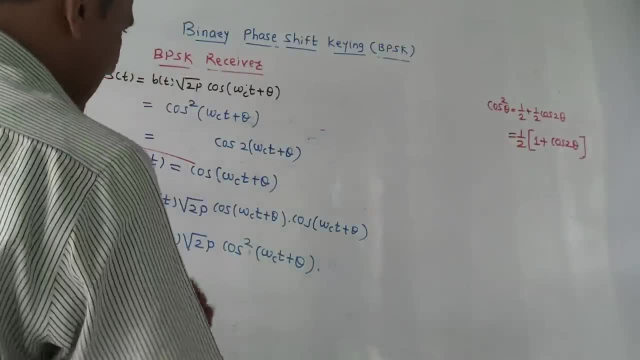 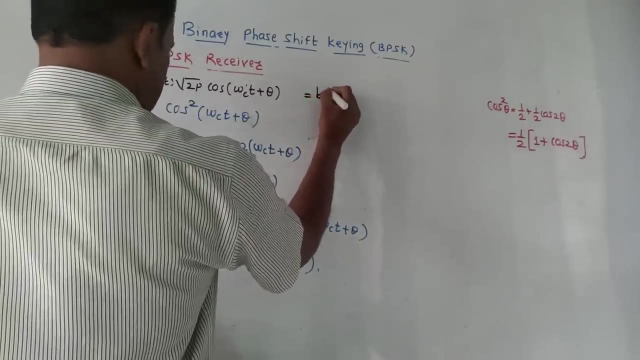 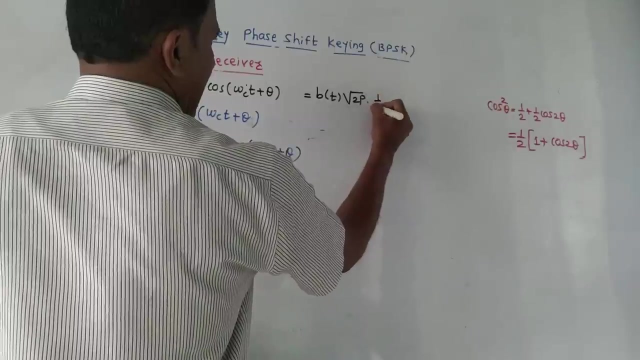 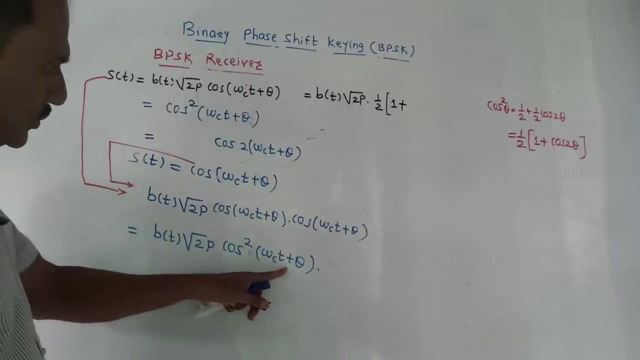 half cos two theta. we can well write this as one half can be taken common, one plus cos two theta. so equation can be written as b of t into root two p. we will cannot write p now looking at it here one plus. it will come here one half into one plus. we are using identity for cos square 1 plus. 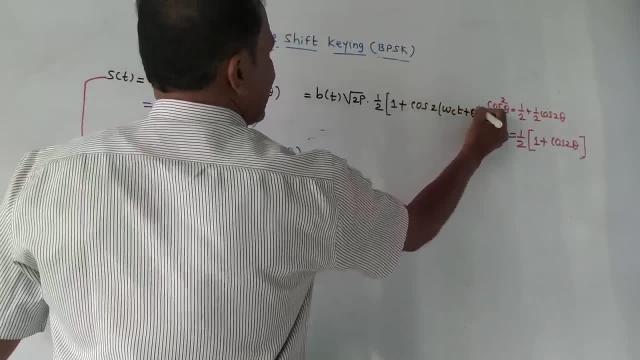 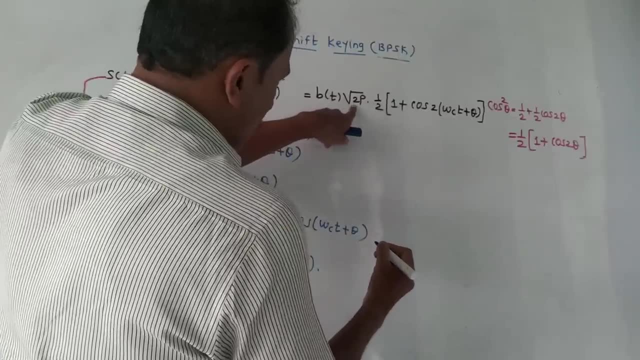 cos two theta, cos two omega c, t plus theta. now looking at one half and we can simplify it. so this is one half and this is root two p. i am not just writing this term for simplicity, but let's say root two p is one half of one half plus one half is root two p. 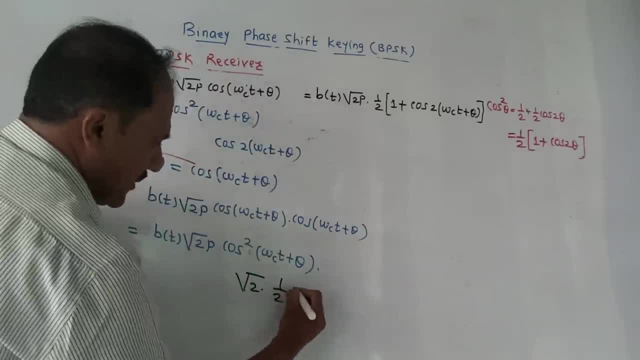 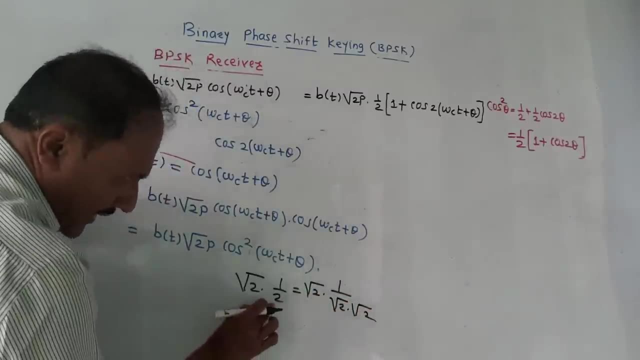 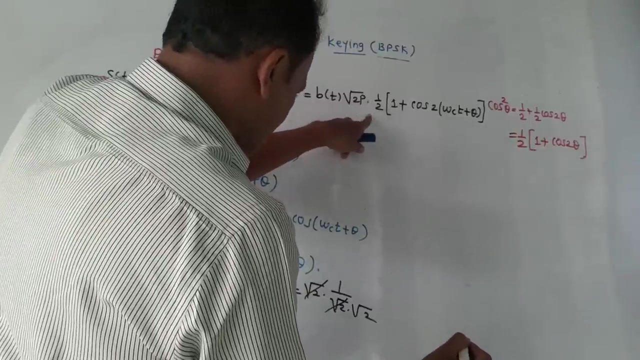 as it is root 2 into 1 half, it can be written as: root 2 into 1 half means root 2 into root 2. yes, here 2 is there in the denominator, so root 2 into root 2. this root 2 will be cancelled. so multiplication of this root 2 and 1 by 2 becomes 1 by root 2. 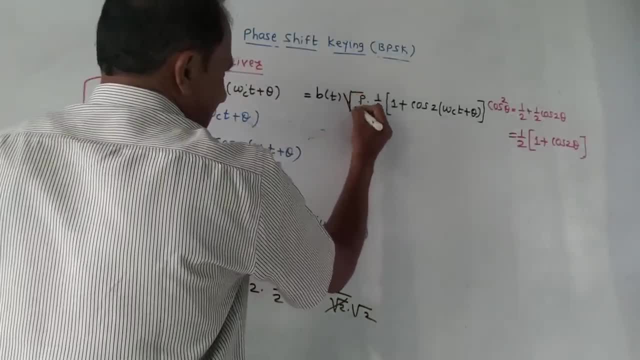 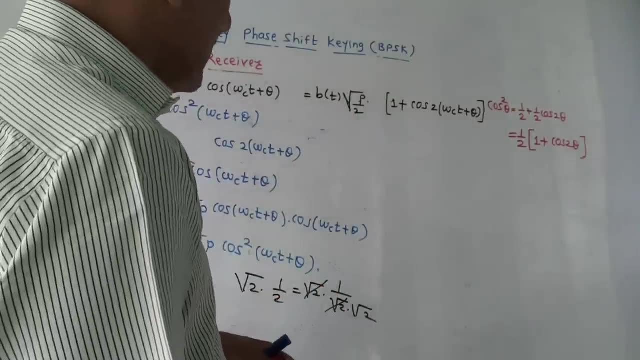 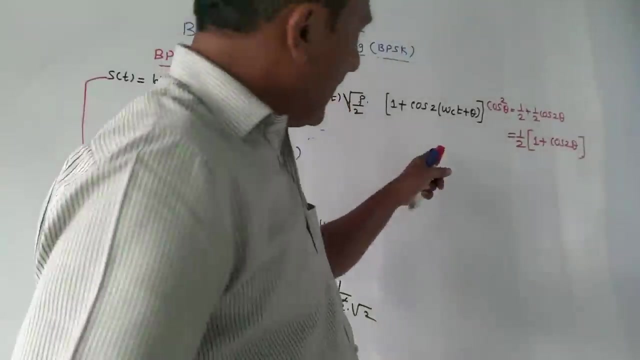 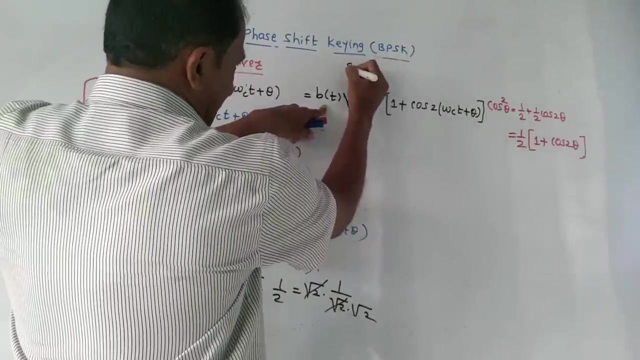 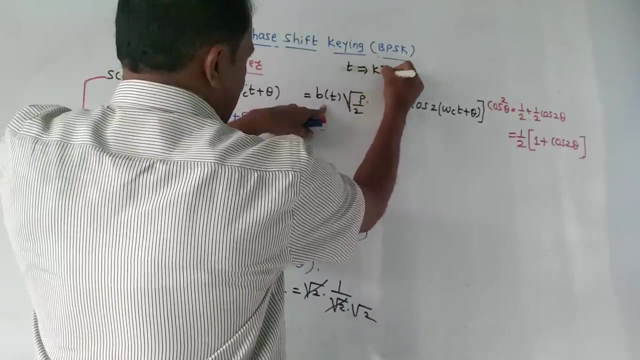 so this equation can be written as square root of p by 2, so I will remove this 1 half according to this calculation. now this signal is applied at the input of integrator, so the next equation. so we will replace, because we are applying it to the integrator. 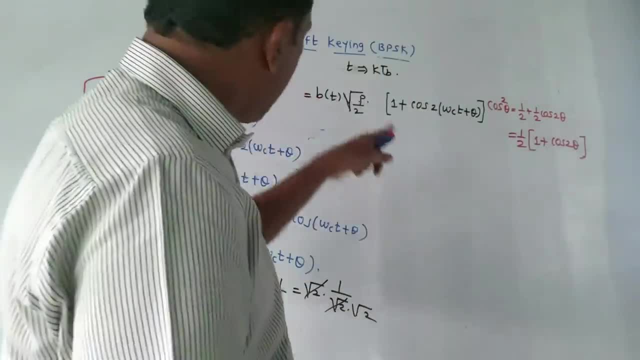 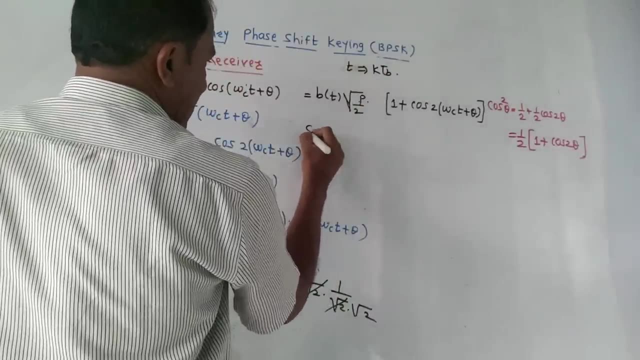 and function of the integrator is to integrate the signal from 0 to or. TB is late. I am replacing K by T, by K TB, so resultant equation can be denoted by s of K TV. yeah, the case of Tiffany is capable of a magnetic s of K. 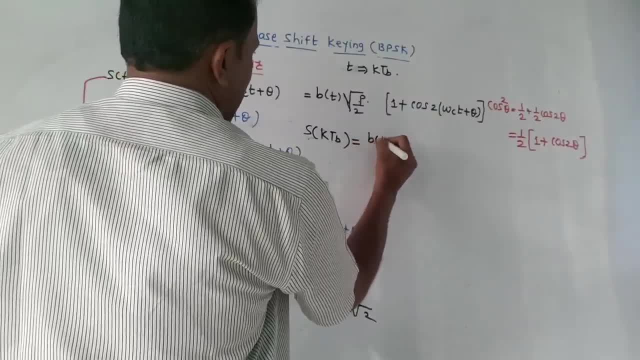 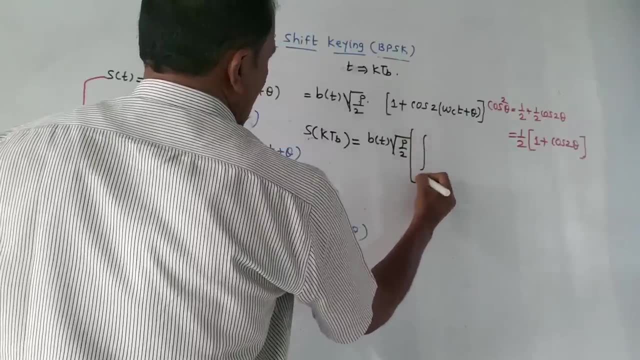 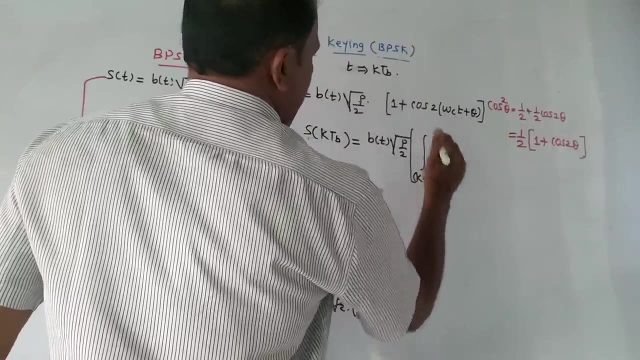 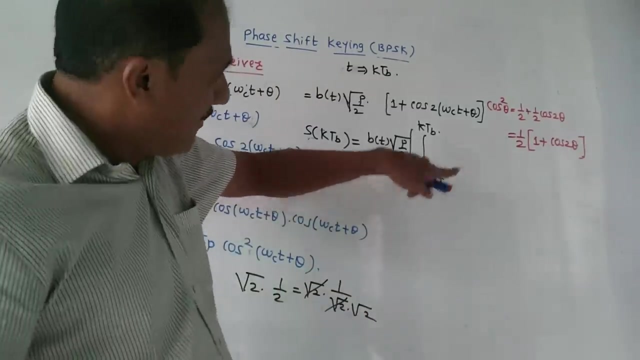 TP. then we will perform integration like this here BT root of P by 2, here constant. to take integration, my select down up, they go k minus 1 TB. k minus 1 TB, say, like a K TV term, actually a poor duration. typically integrate, connect many as I do k, k, k, th bit controller character was kind of a K minus 1 into. 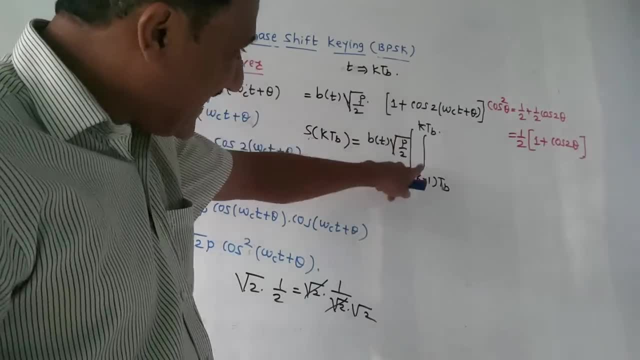 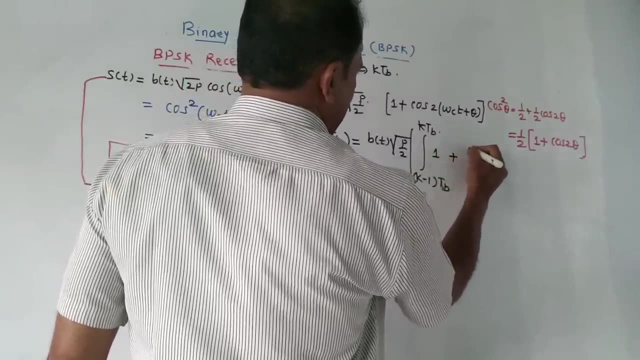 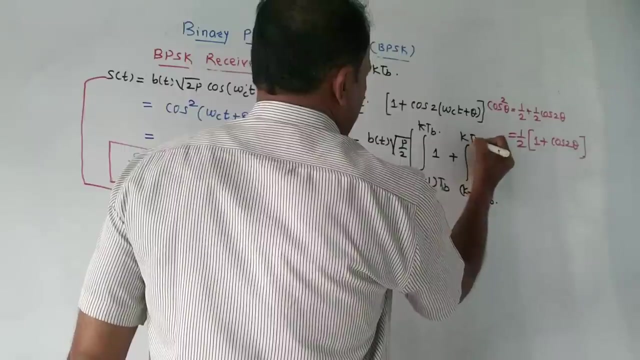 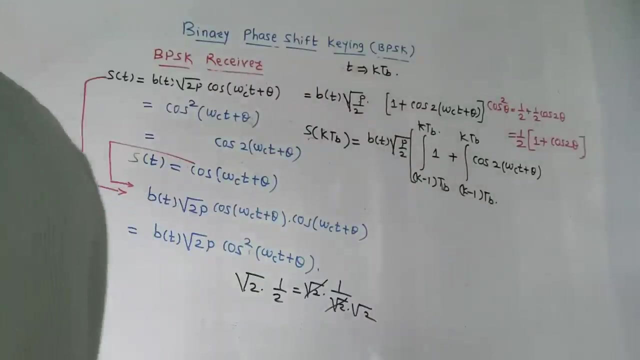 TB up to K TV. so this is the integration for kth bit, first bracket 1 into plus second bracket, though a little bracket. one of them is same integration: k minus 1 TB to K TB, cos of 2, Omega C, T plus theta. up yet though another like integration. 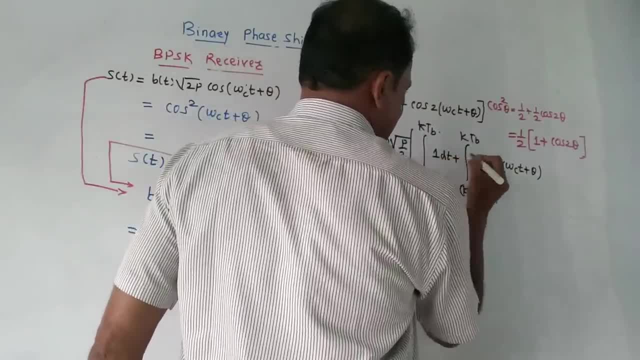 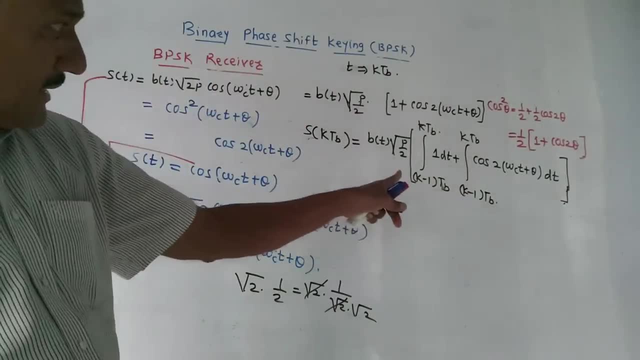 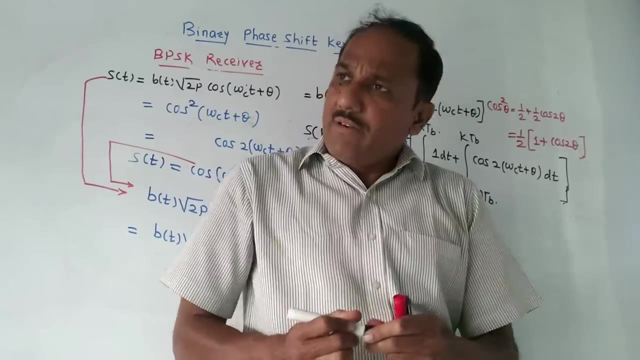 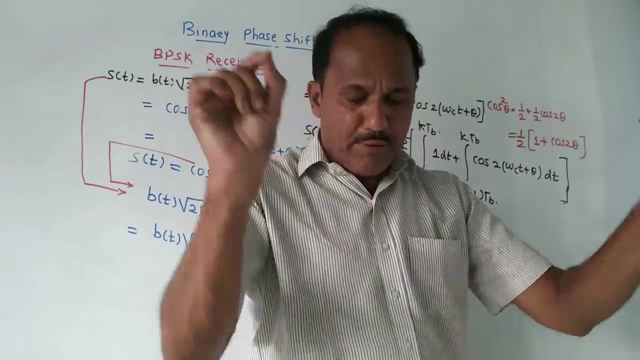 program. look, by default, variable of integration is DT. so you have a big detail. now listen, there are two terms in case of integrator: second term, Joey go- cosine term. I do remember one basic thing in any subject: if you are integrating sine wave or cosine wave for one complete cycle, 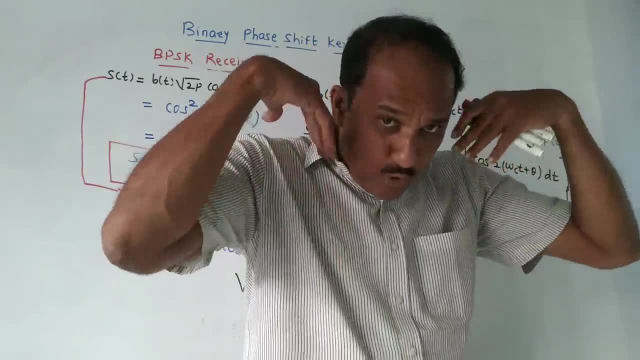 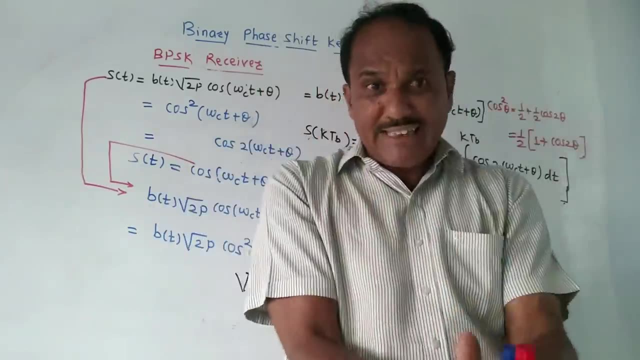 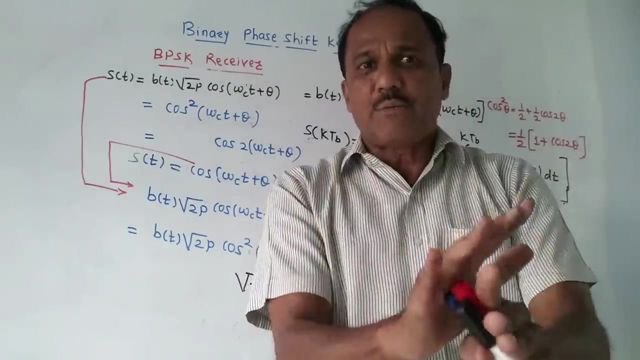 answer of integration is always 0. they go. a poor a cycle kill a sign or cosine wave of integrate career. who to scan, sir Jura, take you key. a poor a cycle, kill a jet. not positive, partial negative portion. I got integration but love indirectly. addition to plus minus become 0. so if you are performing integration for one. 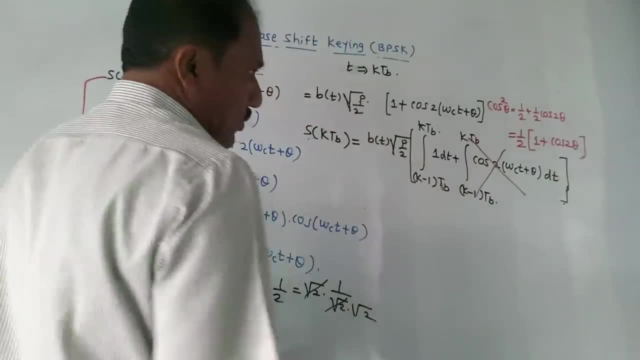 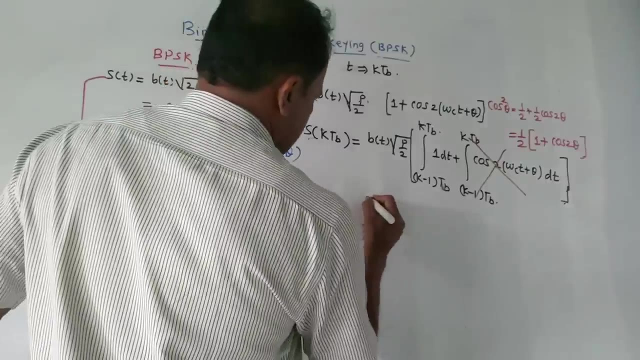 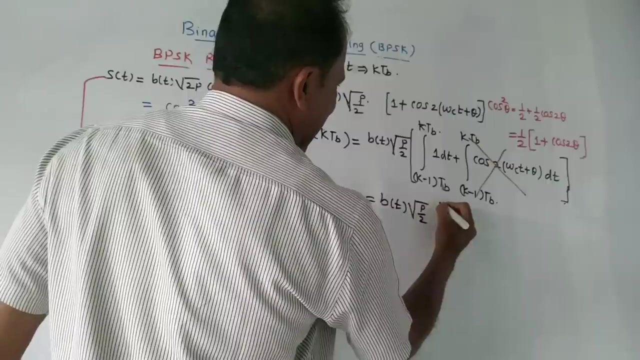 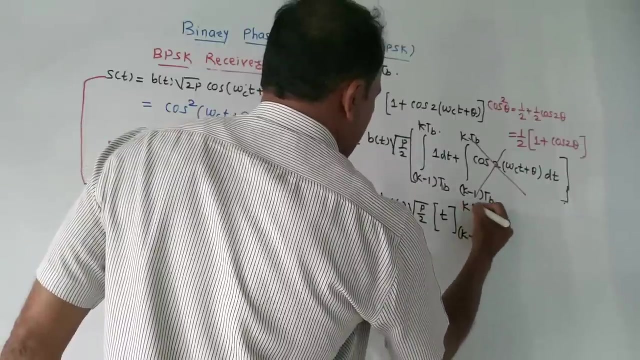 complete cycle and so this term zero. so I'm deleting this term. now for the remaining term. I can write it like this: this is B of T into root P by 2 as it is, yeah, one DT is kind integration T. I got a bar but I mean I select on P limits are K minus 1 TB to K TV. we know. 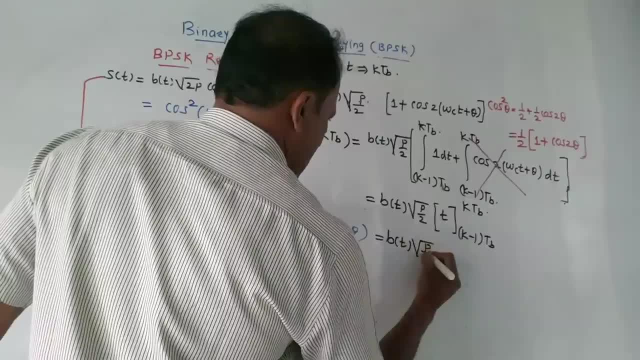 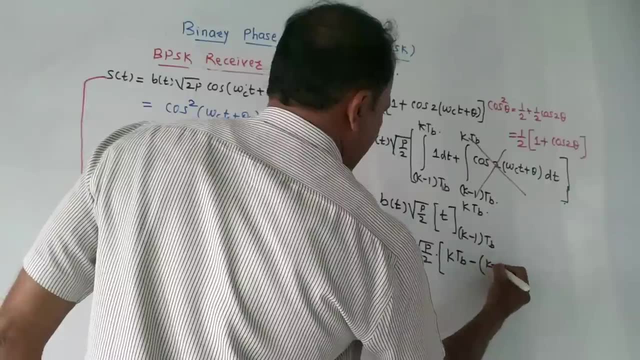 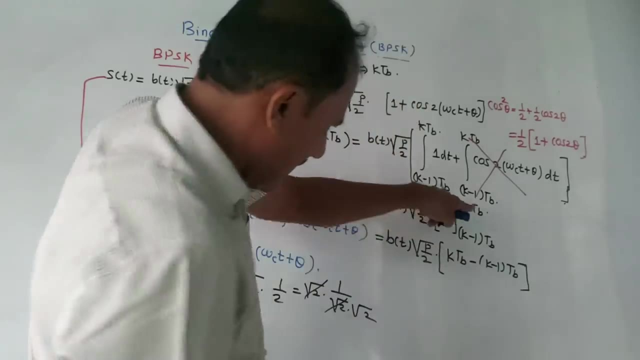 the usual rules of integration. yeah, constant term as it is. laying a pair. a upper limit put. carrying a KTB minus lower limit put. carrying it K minus 1 TV. this is k minus 1 TV. a bar upper limit put, kiya female limit put. yeah, yes, 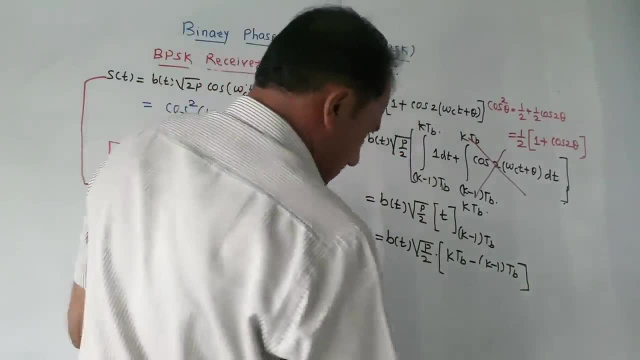 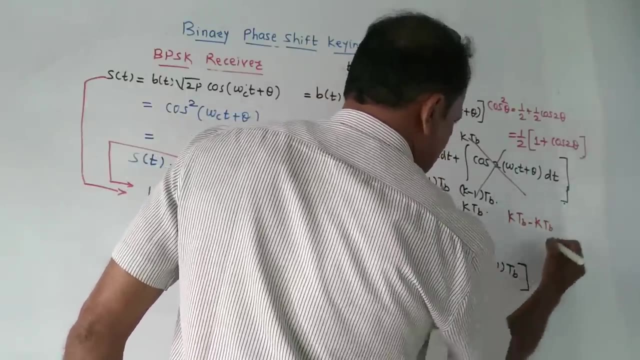 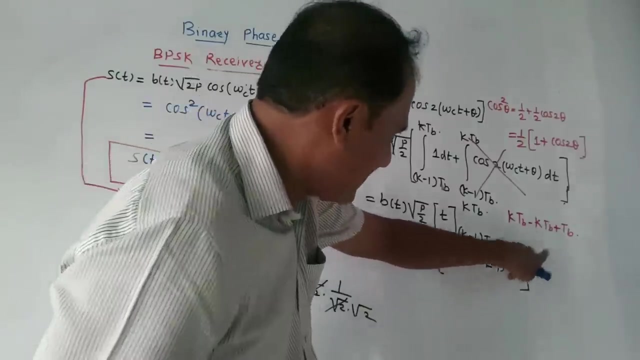 simplify Ukraine. get to simplify current game to is K answer. I gotta go. yes, if yet I'm Alex elected to. KTB minus KTB, or your minus minus become plus plus KP. KTB minus. Whoo. tb minus 1 has become plus plus tb, So this term is cancelled. Its answer is tb, So final. 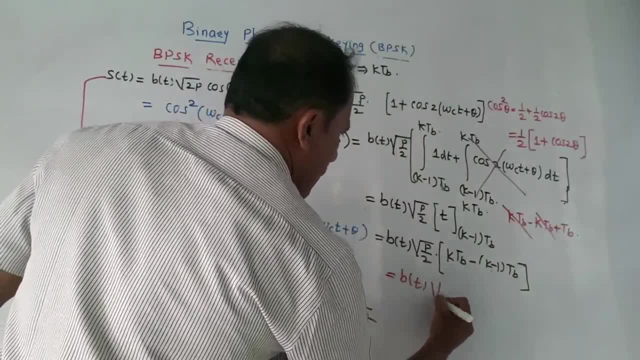 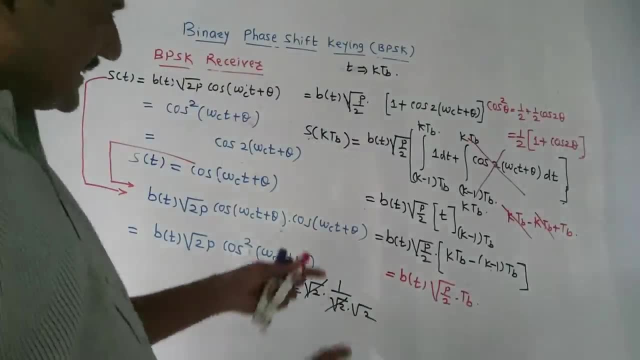 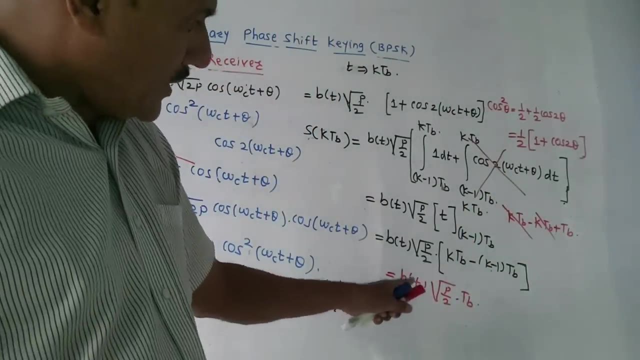 answer is v of t root p by 2 into tb. tb is the bit duration. It indicates that at the output of integrator, whatever signal we are getting, that is directly proportional to the incoming signal. So this is the mathematical expression for BPSK: received signal. 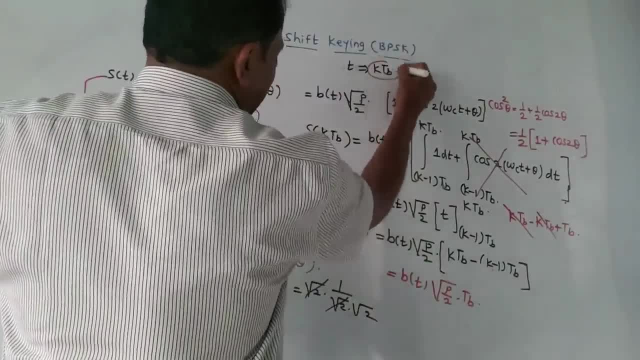 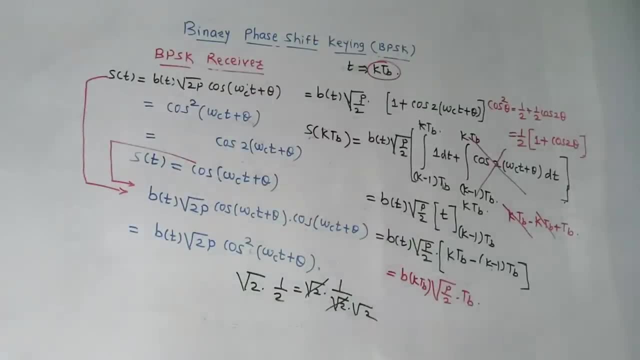 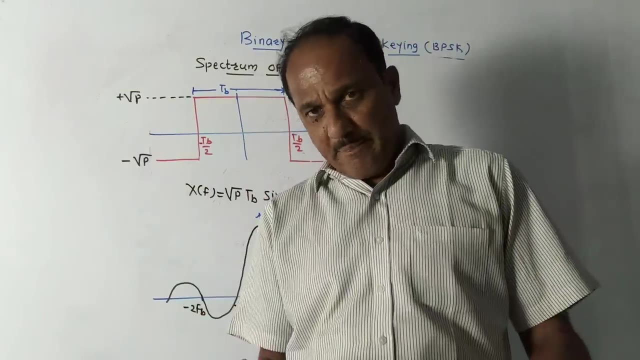 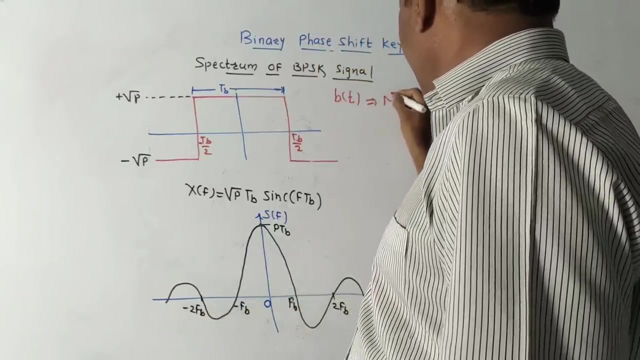 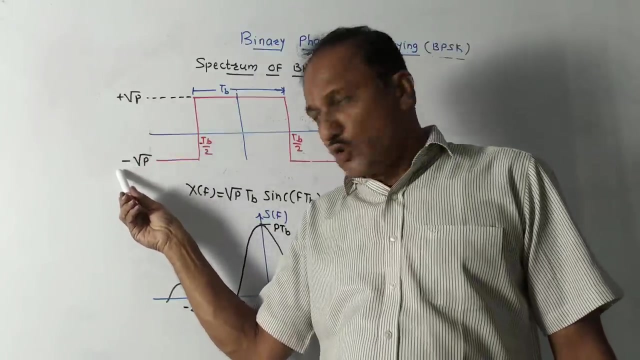 This is the final expression. Next part is spectrum of BPSK signal. In BPSK the signal v of t is bipolar, n r, z, non-return to 0. So its maximum amplitude is root p by 2 into minus root p. Minimum is minus root p And its width is minus tb by 2 to plus tb by 2.. 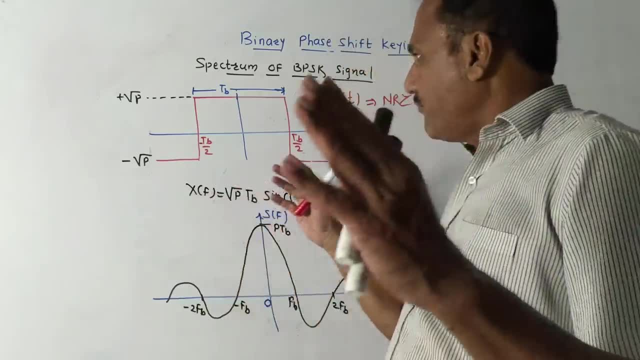 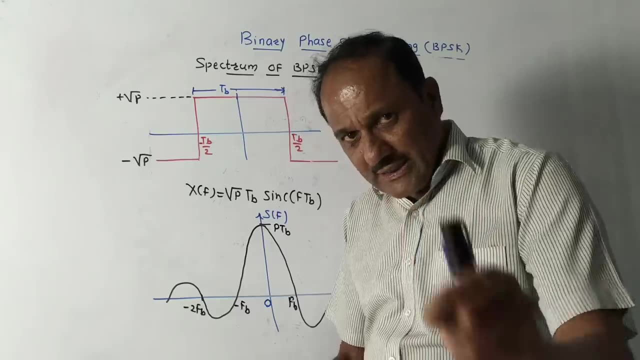 Now, spectrum means Fourier transform. You don't have to mug up the lengthy formula as far as this part is concerned. Remember a basic formula: Fourier transform of rectangular signal is a sinc function. This is basically a rectangular signal, So directly we can. 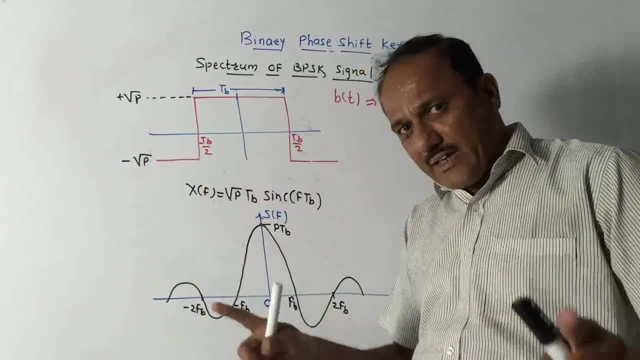 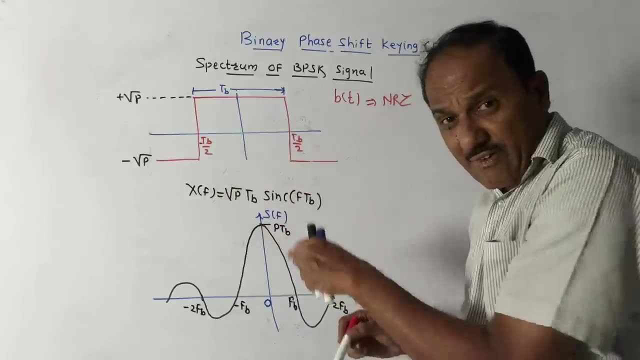 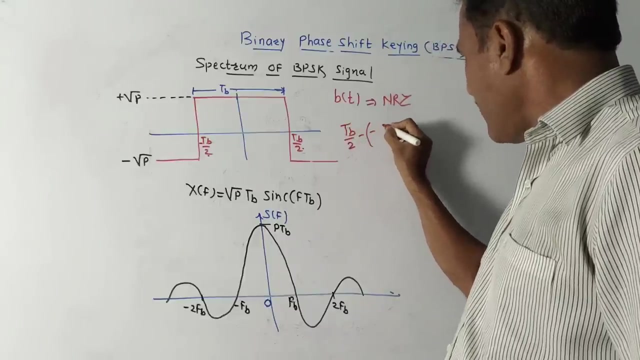 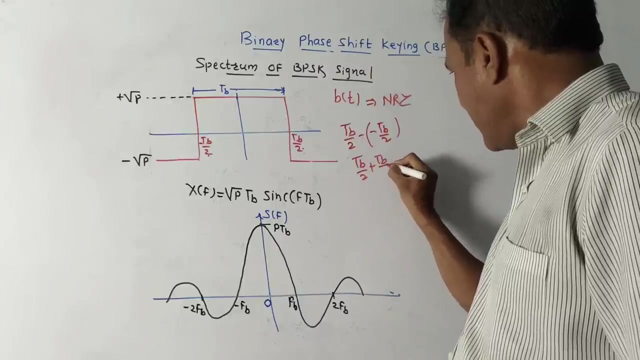 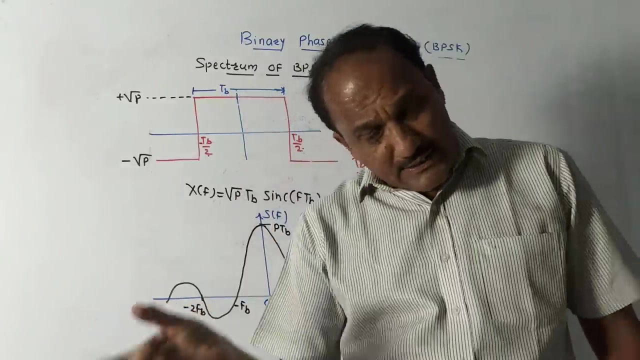 write the equation of spectrum means we can write the equation of Fourier transform. Million should be written at the x-axis. The written humanities of s are regular, But it might be used forетime time. suppose we should write it for the sum of s as 0, r, x, z. That is really not necessary as the equation may not be taken, So this: 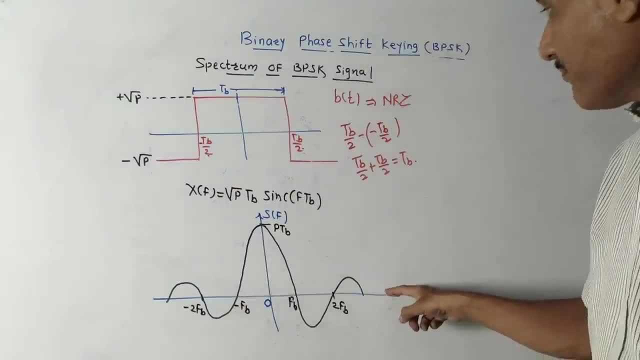 is basically only a linear expression of spectrum. The lineרהwd is spin-Wo, g справ is infinite. See in the diagram written instead of time. edges is a line. The line would have been cot Prime by 5 meters. The second: consider. this time we will see that 1 is usually 1.5mx. 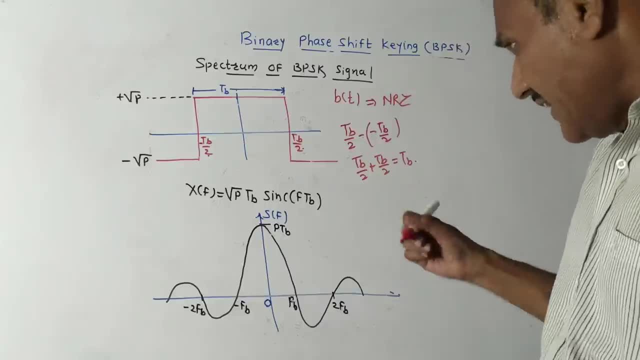 which is 1.5m x YES. in a given time it is 1.3m x BPSK is 1.. Fine, it is So the difference. Now see, this is a SYNC function, so how to write its mathematical equation.